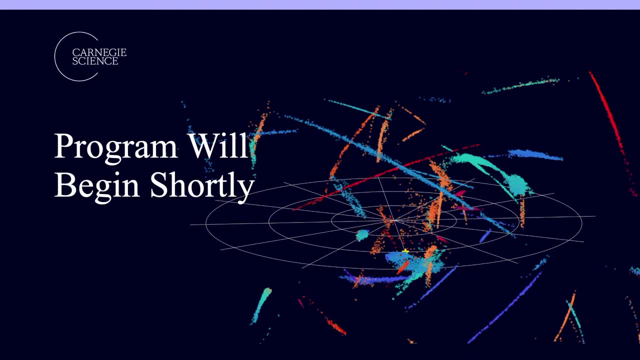 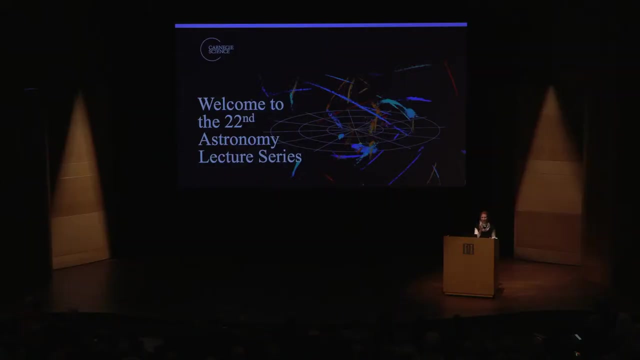 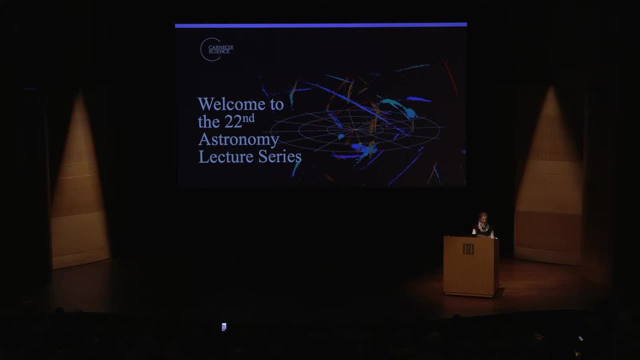 Thank you for watching. Thank you for watching. Thank you for watching. Good evening For those of you who arrived a few minutes ago. welcome to the 22nd season of the Carnegie Astronomy Lectures. Since 2003,, these have been one of our most popular public programs of the observatories. 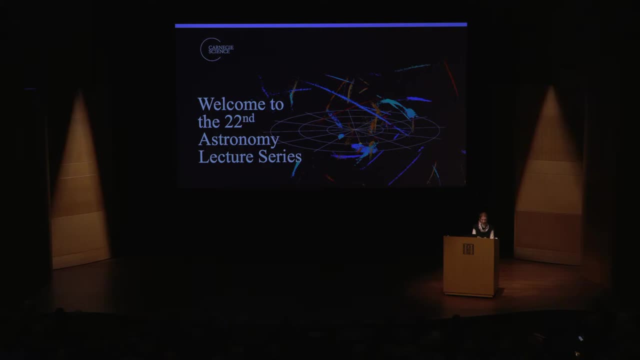 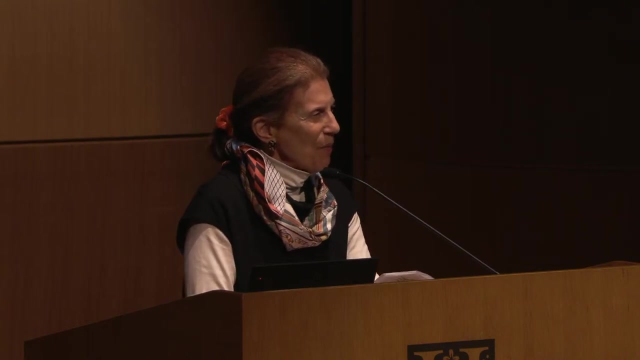 And it's a great pleasure to see tonight's large and loyal turnout. And a special welcome to those of you who are also streaming this lecture from home or wherever you may be. One of them may be our director, Dr John LaValle. 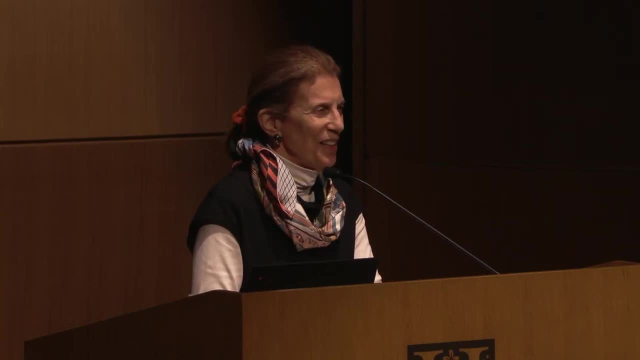 John Mulcahy, who is in Dallas, along with several other Carnegie staff, in preparation for the eclipse next Monday, with fingers crossed for the weather, but that's another subject. Anyway, as you know, these programs are created by Carnegie Observatories, which is the oldest. 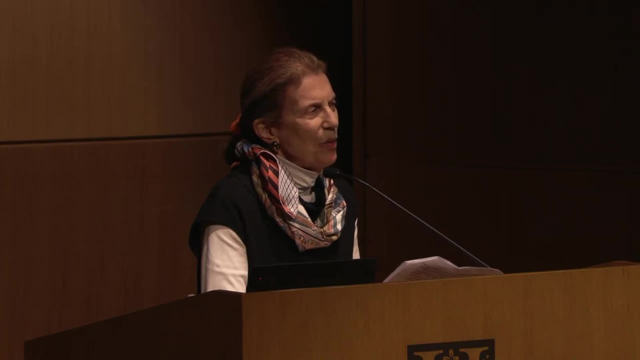 scientific organization in Pasadena and probably the oldest in Los Angeles- I mean in Southern California, not just Los Angeles, but it was founded in 1904, and today is one of the world's destinations for contemporary research in astronomy and astrophysics. 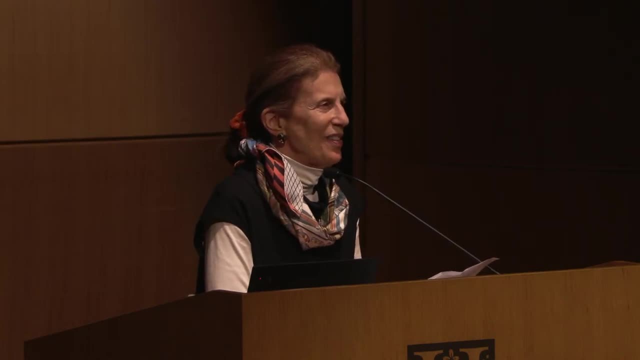 It's also great to be back at the Huntington, which has been our home for this series since practically every season. The Huntington holds all of the Carnegie's historic papers and is a splendid partner with us. I'd like to give special thanks to two of our wonderful colleagues here, Kimberly Feeney. 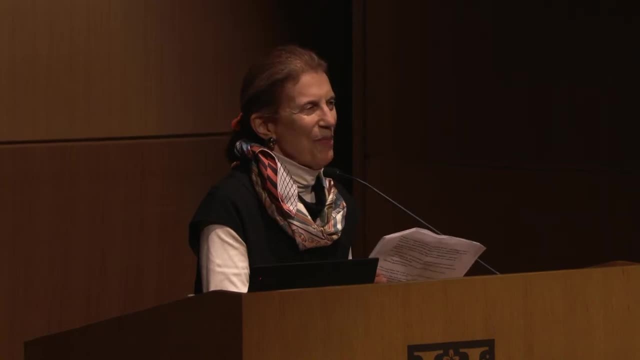 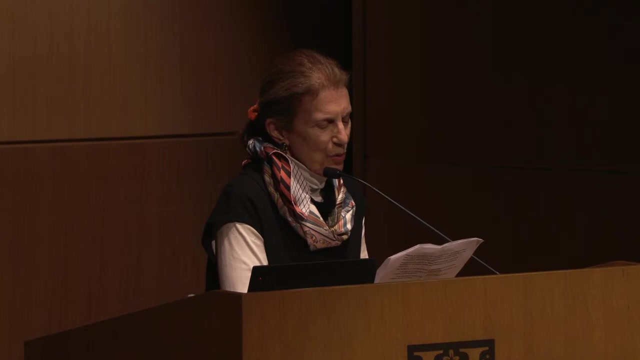 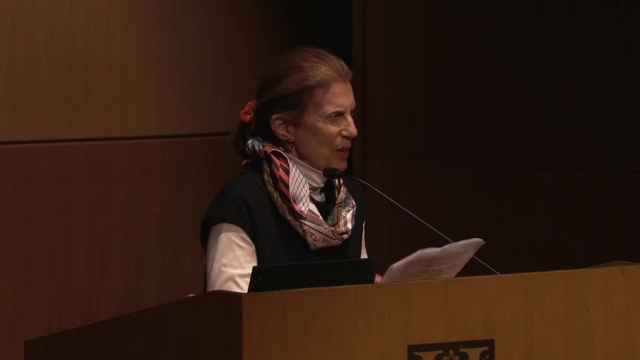 Following tonight's talk, everyone will have the opportunity to ask questions. There will be microphones at each of the two aisles. If you haven't already done so, please turn off or silence your cell phones. Now to tonight's speaker. It's an honor to interview him. 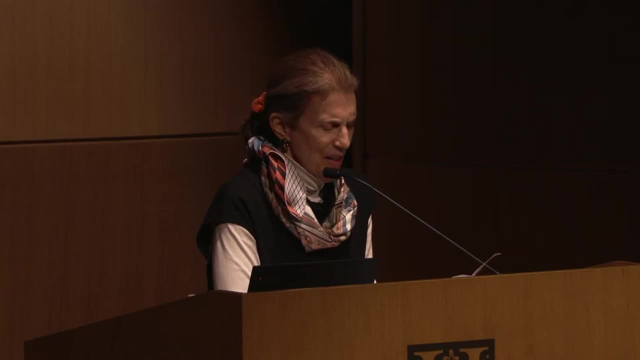 introduce Dr Anna Bonassa, a Carnegie staff scientist and one of the top young astronomers truly in the world today. Prior to coming to the Carnegie in 2021,, Dr Bonassa was a fellow at the Institute for Theory and Computation in the Harvard and Smithsonian Center for 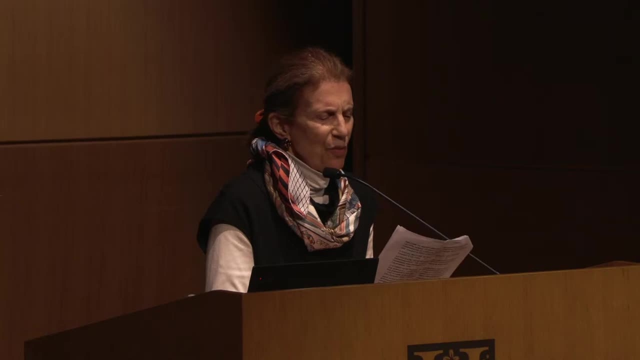 Astrophysics. She received her PhD from Yale and her Master of Science from the University of Zagreb in Croatia. She's the recipient of many awards, including the Warner Prize in 2023, which is the top award for young astronomers, and the Brouwer Prize for her. 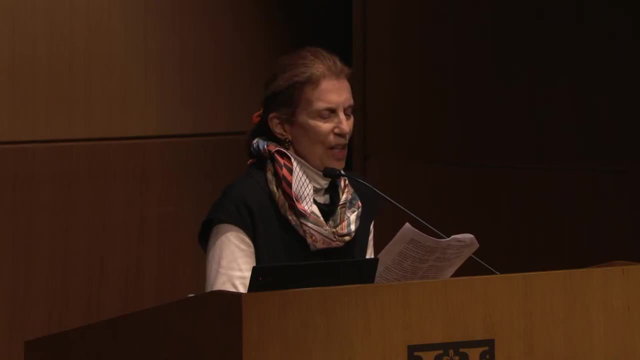 PhD thesis at Yale. among many others, She's been the lead author or co-author on 53 scientific papers to date. Currently she's also heading something called the VIA Project, which is an all-sky survey of the Milky Way halo, which I'm sure you'll hear more about And like. 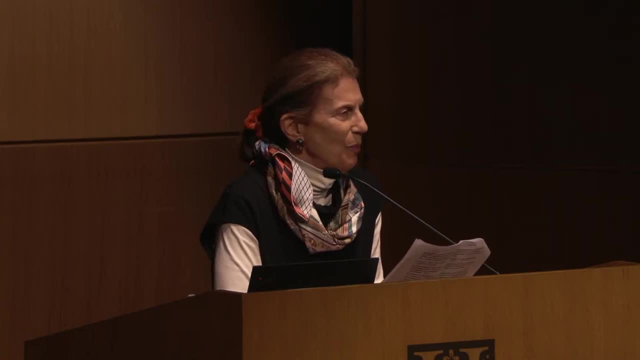 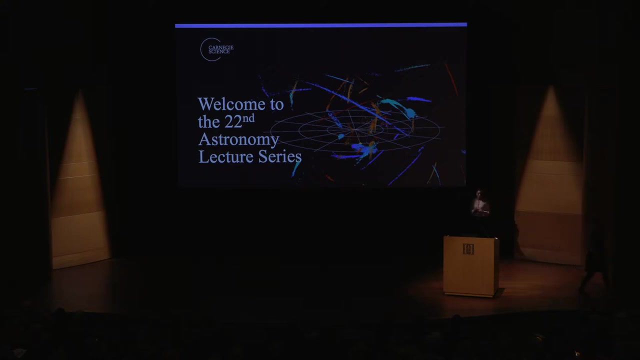 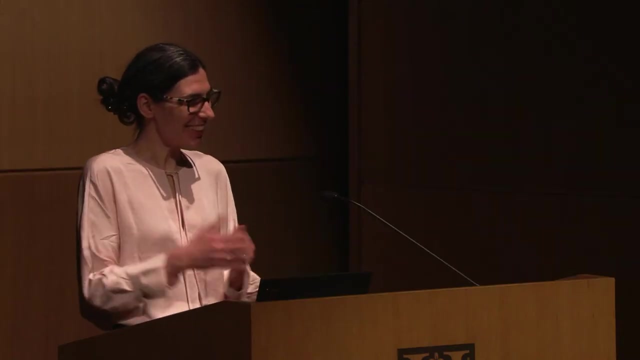 many of our Carnegie astronomers. Dr Bonassa is extremely involved in education, Education and outreach from graduate and undergraduate students to K-12 programs. Please welcome, Dr Bonassa. Thank you all for coming. I'm excited to tell you about dark matter. We do think there is. 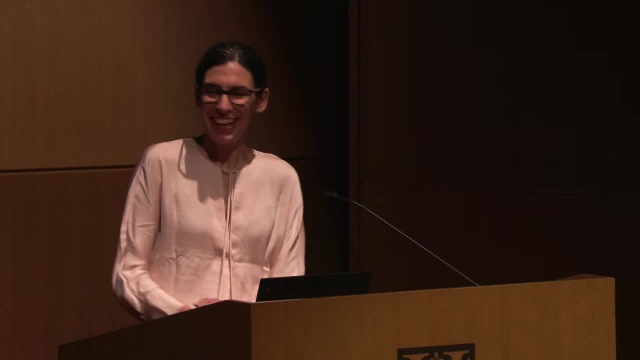 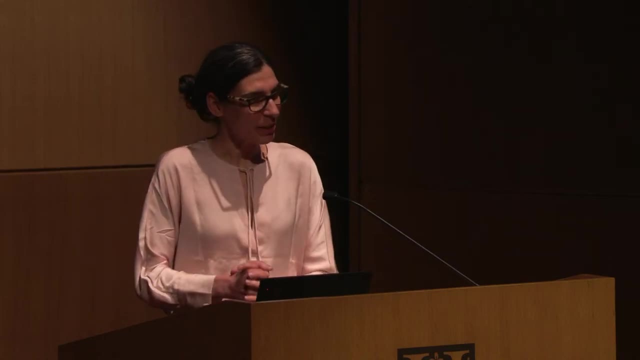 dark matter and it makes up 90% of our galaxy. Thank you, Thank you. This image is very much from a large兄, totally galaxy. What I'm showing here in the background is the view of a simulation from a former Carnegie postdoc called Andrew. 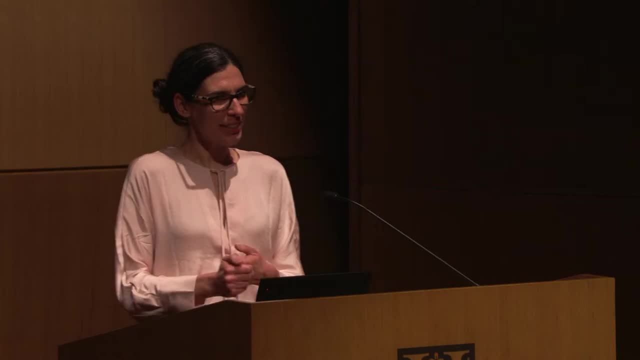 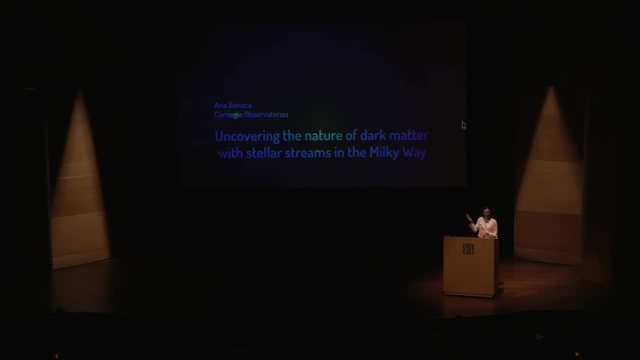 Wedzell, who is now faculty at UC Davis, And this is still one of the most realistic numerical computer simulations of a Milky Way-like galaxy. You're seeing here is dark matter which you think makes up almost 90% of everything there is in the Milky Way. 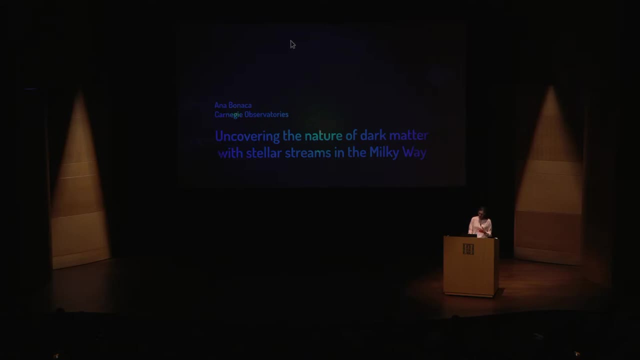 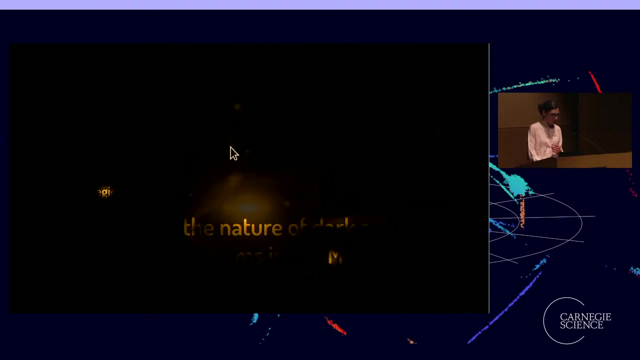 inner part is where kind of all of the stars are, but they are surrounded by a massive halo of dark matter. What we see is looks like this: So still, there are some stars in the simulation. there are some small groups of stars around, but this is only 10% of the 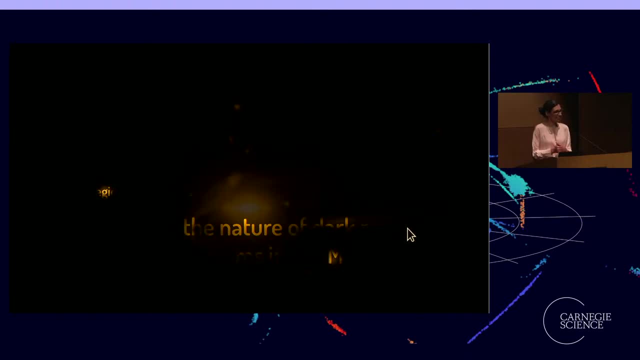 information And, as you can see, this title slide is not super informative if you're only getting 10% of the information that there is in it. So, yeah, we don't really know what dark matter is, and other than just being very curious about the universe that surrounds. 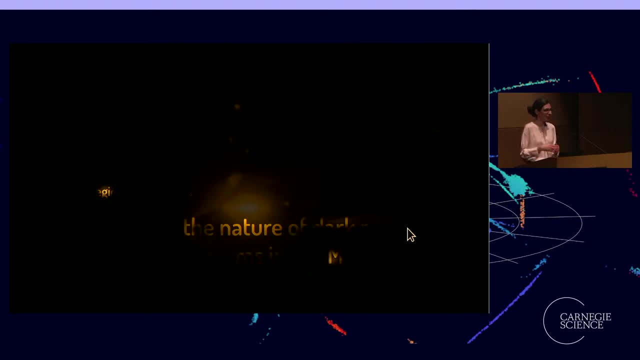 us. we think it might be important for actually understanding everything and how it came to be. So why do we think there is dark matter? Well, the answer is gravity, And so Eric warned me to tread lightly with the graphs, but she didn't say anything about equations, So I decided to sneak one in. 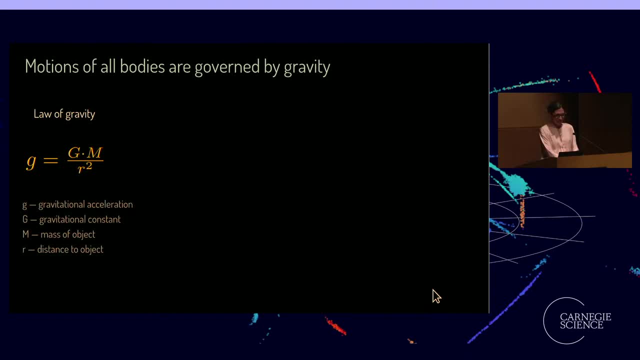 It's a really big, important one. So this expression shows the how we can calculate the gravitational acceleration And so, and this is, the lowercase g equals the uppercase g, which is the gravitational constant times the mass of the object. that is kind of attracting. 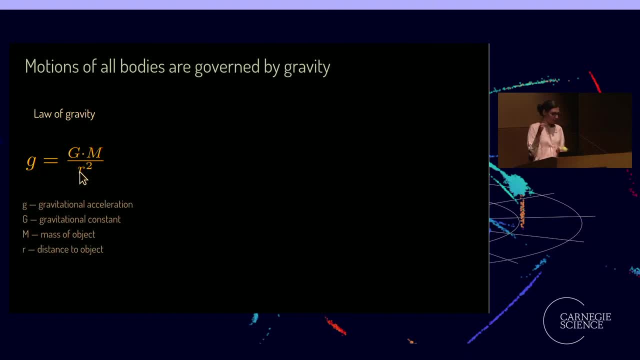 us and then our distance squared to the object in the denominator, And so this is a really fundamental equation and how we came to know there is dark matter and also what, how we hope to learn more about it is An important part. is that this, really only this expression? 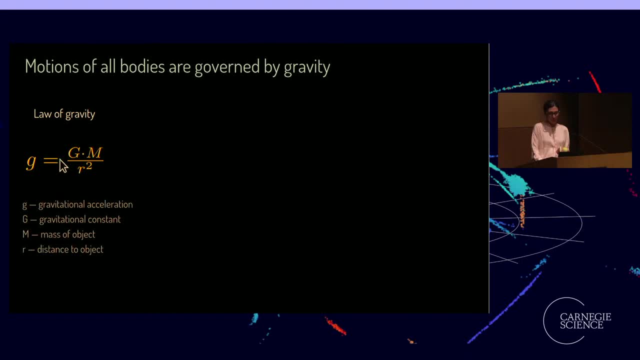 only has two big properties, So the, The, The, The. You know that capital G is the constant, And so it only depends on two parameters: One is the, the mass, and the other is the distance to the object. and so I have here: 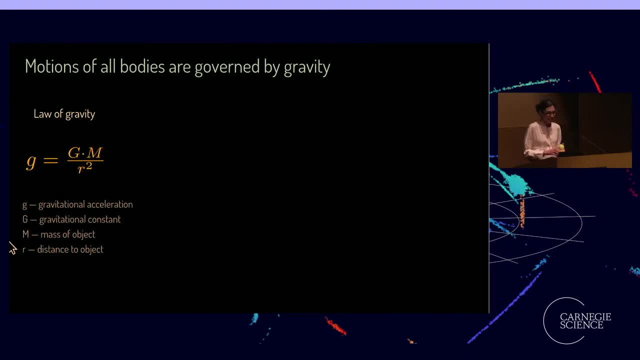 Okay, I'm going to lay it over here. I have a brief demonstration following something that you may have seen in other places. I have two objects- a ball and a packet of of tissues, and if I drop them, they fill up. 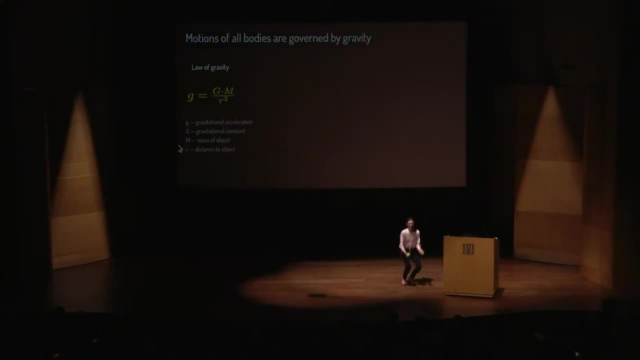 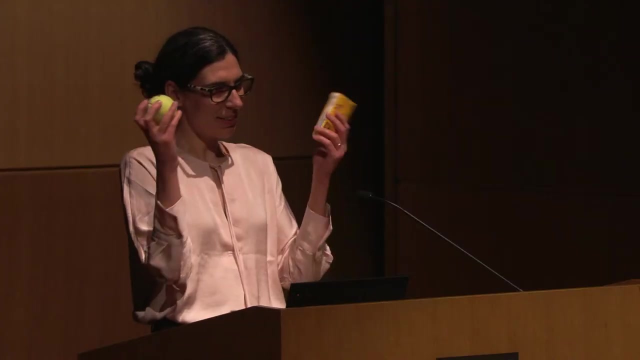 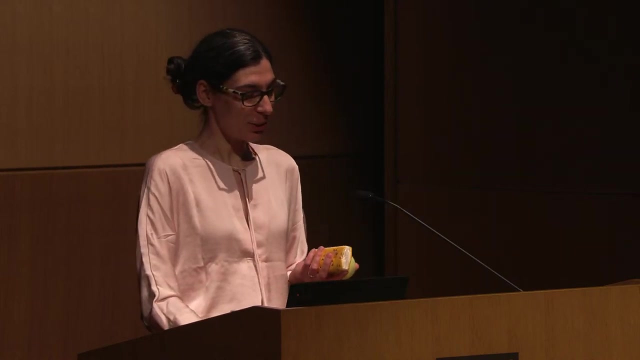 They fell at the same time. Why? Because, even though they are very different shapes, they have different masses, they are different themselves. However, they are feeling the same gravitational acceleration from the Earth, So the mass of the Earth is the same for both. 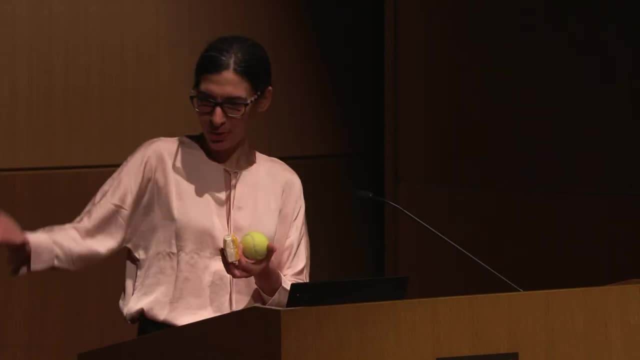 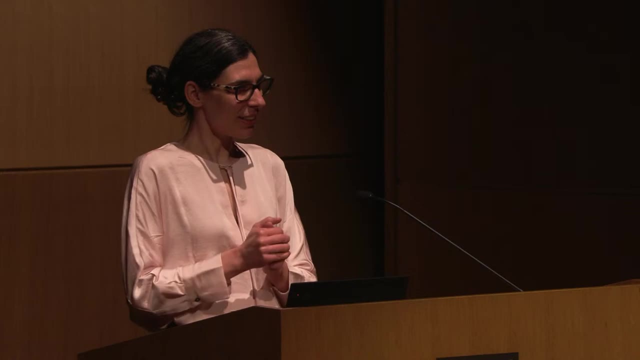 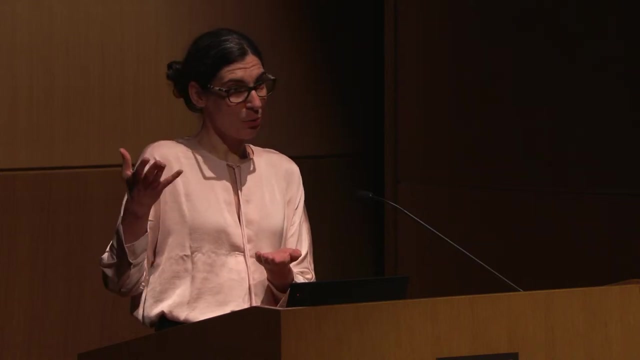 objects, and the distance to the Earth, to the surface, is the same for both objects, So this means that they move the same way, And so one of the deep insights that happened in the 17th century is that we can use this knowledge of how objects move on the surface. 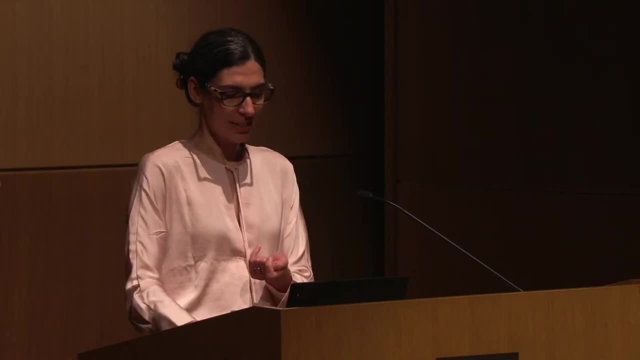 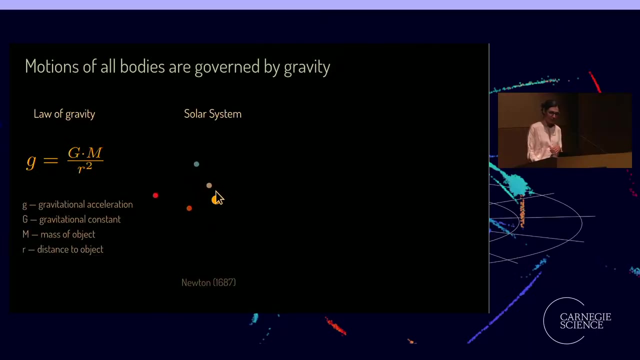 of Earth and apply them to the motions of objects in the sky, And so here I have a graph of planets orbiting the Sun. So the central circle is the Sun, then Mercury, Venus, Earth and Mars, And you can see Mercury moves. 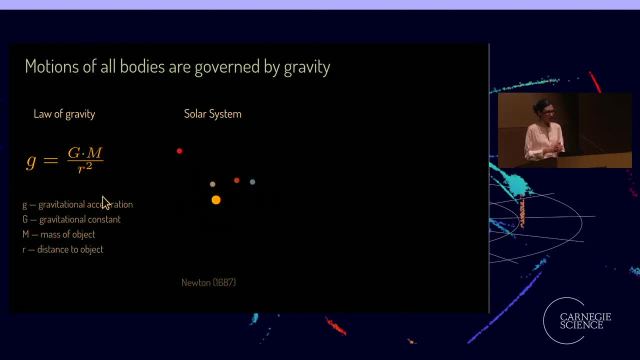 pretty fast around the Sun, Mars not so much. We can exactly explain this with this equation: The mass of the Sun, which is attracting all of these planets, is the same, but their distances are different, And so, if we were to plot plot alert, we have rotational velocity. 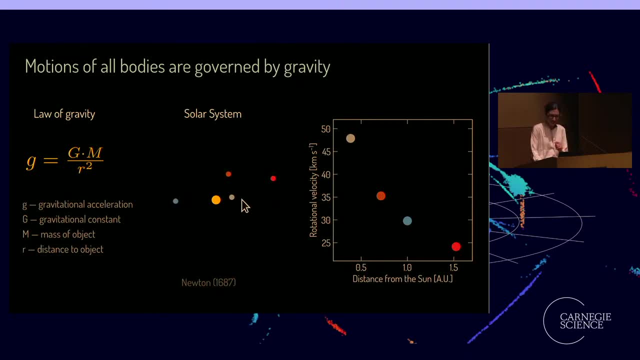 I color coded the points the same way so I can map them one to one. We see as a function of distance to the Sun. Also, we see that the highest velocity is for Mercury, which is the closest, and then it falls off rather steeply, And so this was a really successful model. It explained. 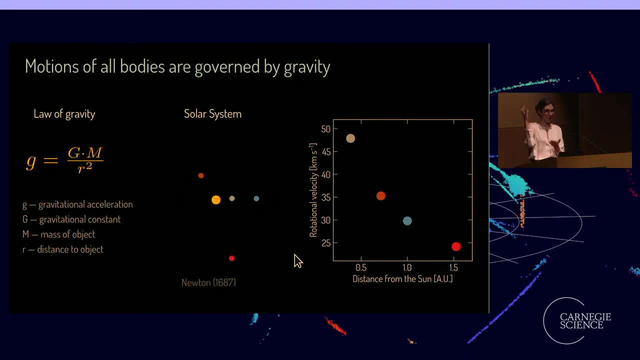 how objects move and can explain how planets move in the night sky. It was so successful that there were even some irregularities noted in the motion of planet Uranus and people hypothesized that there must be another planet. Brig Vishal whirls. consumer device carrier. 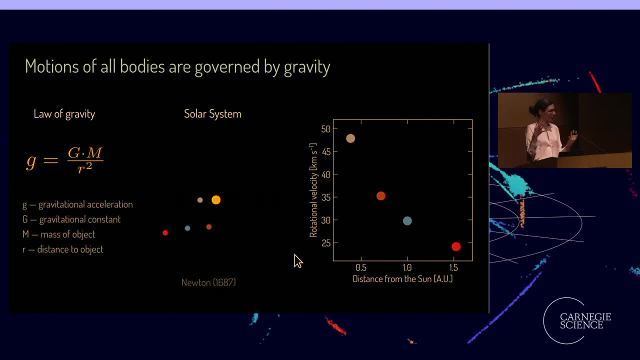 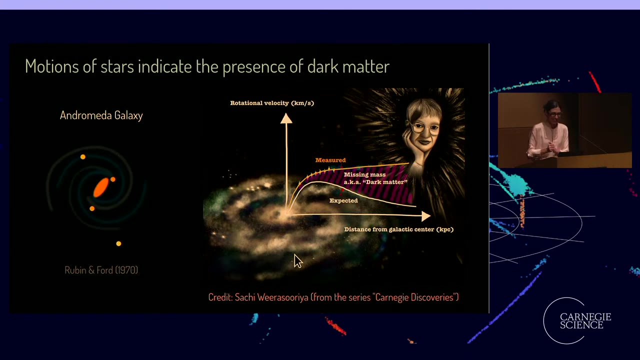 outlining probe And predicted where the orbit of your planet should be And many that are considered salvатели should be, and led to this successful discovery of Neptune. So this was like all good and it's really a very successful physical theory. So it was great, Except when we kind of branched out And so here 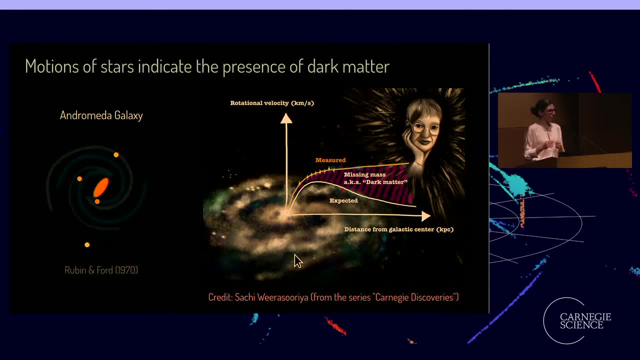 I'm showing a work of Vera Rubin who measured motions of stars in the Andromeda Galaxy, And so in this cartoon you can see that there are again four points, the nominating stars, And they're all moving pretty fast. So this outer one is not quite as slow as Mars was in the previous slide. 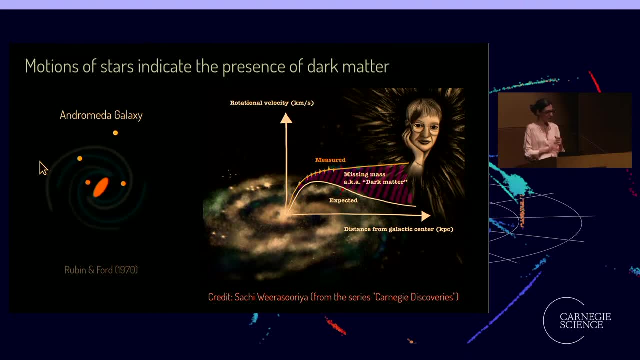 So this was unexpected because we thought, okay, if all of the mass is in the stars that we see, then the outermost stars should be moving much slower than they do, And this is depicted here in this very nice graphic from one of our current postdocs, Sachi Wirasuriya. 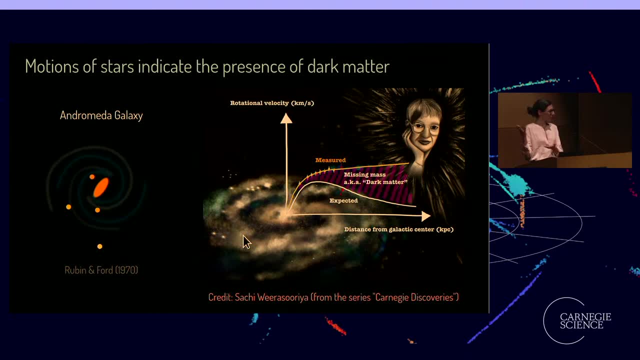 who is not just a scientist studying dark matter herself, but also very interested in science illustration. And so here she depicted the discovery of Vera Rubin, who was Carnegie astronomer and shown the measurement of rotational velocity on the y-axis as a function of distance from the galactic center on the x-axis. And so what was expected was one of the stars moving faster than they do, And so what was expected was one of the stars moving faster than the galactic center on the x-axis, And so what was expected was one of the stars moving faster than they do, And so what was expected was one of the stars moving faster than they do, And there. 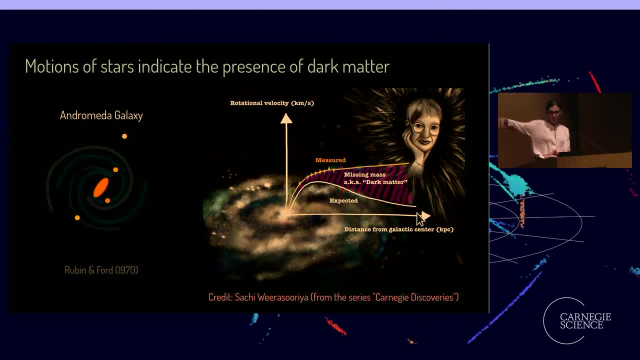 are sort of enormous curves, that kind of falls down. as we go to larger distances. we expect that the stars being moving slower, but she actually measured is that they remain pretty, pretty fast. And this discrepancy is what we call dark matter, And there appear to 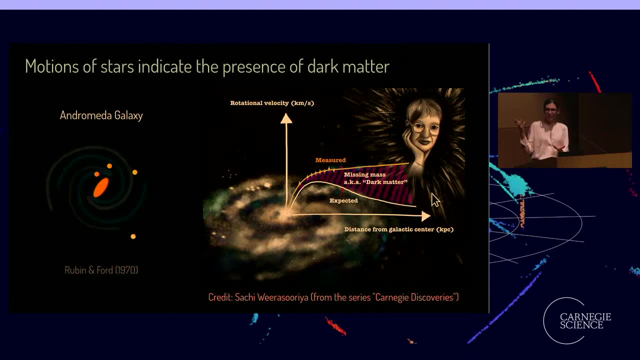 be quite a lot of it, And we don't see it here on Earth. This was really like the phenomenon that we see around galaxies in the sky, So then people started wondering: okay, can we learn more, more about dark matter from properties of galaxies? 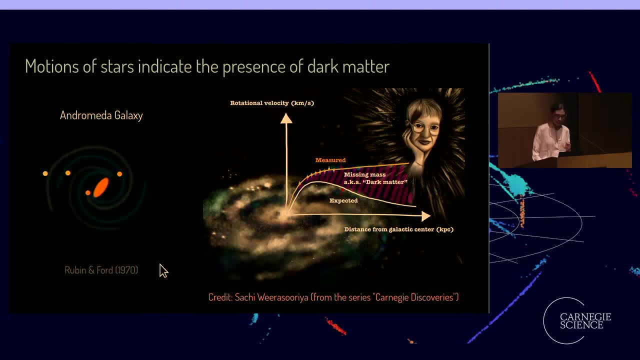 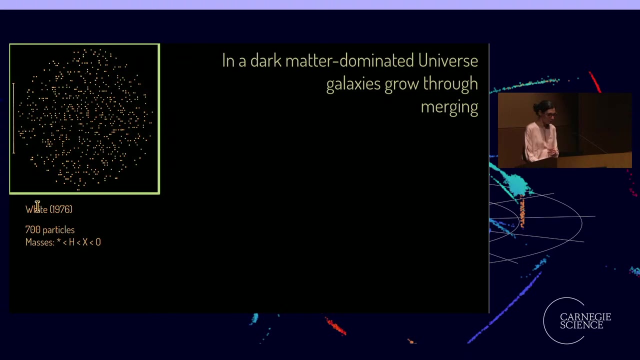 And so this was a discovery that was made in 1970. And kind of in the next few years after that. people started to run calculations either on paper or on early days of computers, And one that I found really interesting was here from Simon White in 1976,. 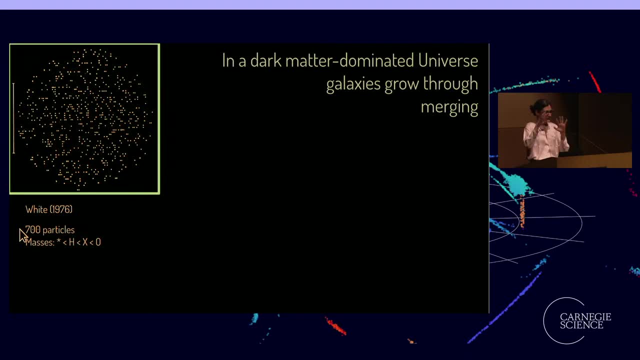 that had 700 particles of different masses that represent different galaxies, And then just the calculation was to calculating basically the gravitational forces between each of the pairs of these particles. And so, as time went on, what Simon noticed it does that the more massive particles 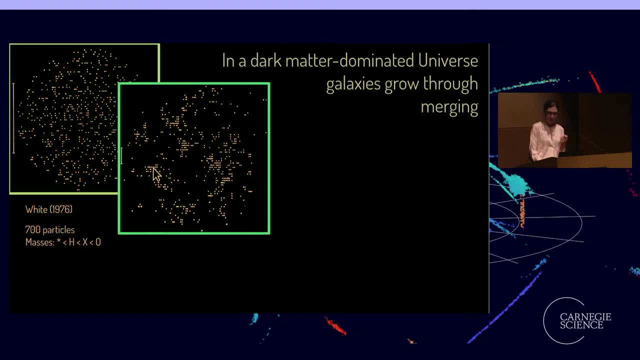 kind of attract the other ones, producing such a clustered structure And kind of goes on until they're like two very massive, massive objects over here, And then the final snapshots. they kind of all get together in this very kind of hierarchical sense where the most massive objects 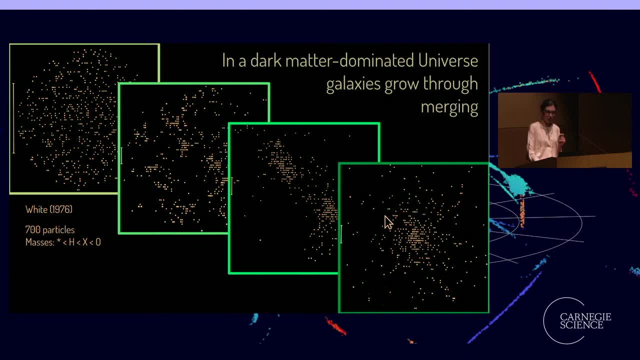 are kind of close to the center and there are some less massive objects in the outskirts, And so this was a prediction of this theory. If there is dark matter and it's so common around the universe, then galaxies should be growing, not just on its own. 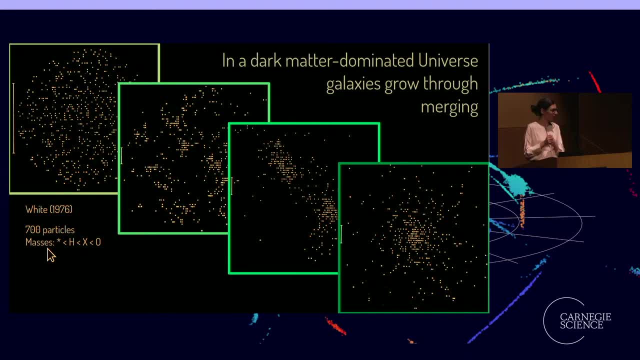 but actually by kind of ingesting smaller galaxies. So this was great, because we finally had a prediction and wanted to know: well, is this really what happens for galaxies in our universe? If so, then it would mean this theory is probably correct. 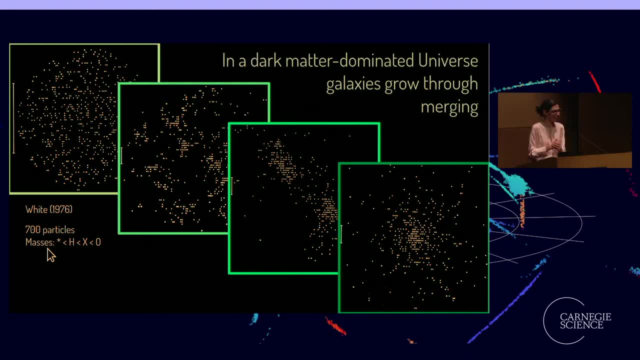 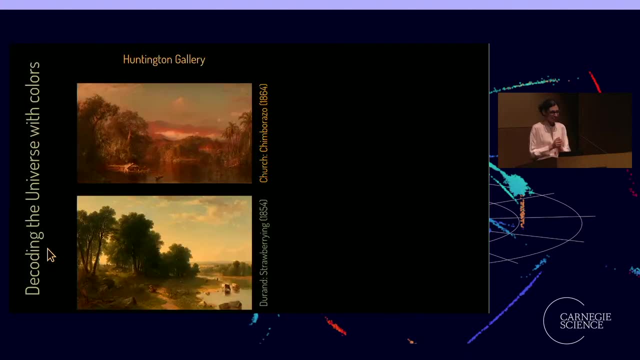 or it checks out. So how do you do that Turns out? yeah, we'll need to take a small step back And, yes, take clues from color. So I have here a couple of example pictures from the Huntington Gallery that some of you may be familiar with. 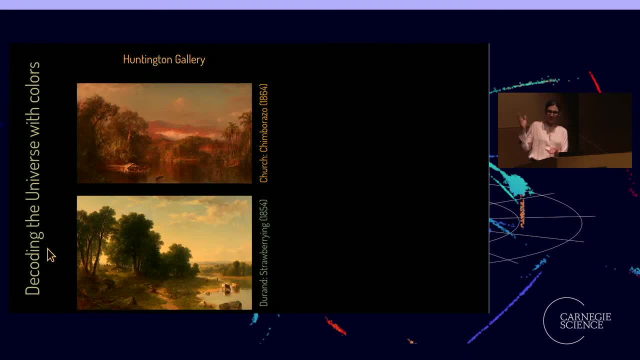 Both are landscapes, but they're kind of very different in tone. So this is meant to show that we can still pass a lot of information in true color. So when you see the top one, which is kind of in reddish tone, 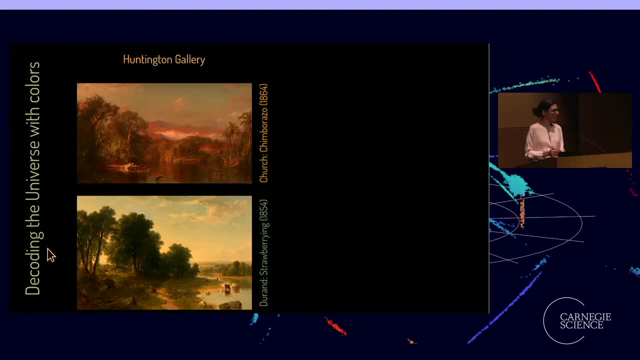 what does this suggest to you? Sunset, So a special time of day. Anything else, Or heat, Or heat, Yes, Again, more temperature. Anything else, Sorry. Wave one, Wave one, Light wave one, Light wave one. 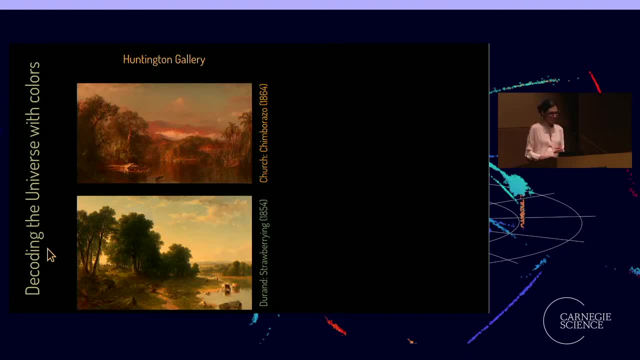 A little bit more red, Yeah. What about the blue one? Clear, Cooler, Cloudier, Anyway, there are some like variations People do. yeah, there is, everyone has their own perception, but the main point is that we can pass some information. 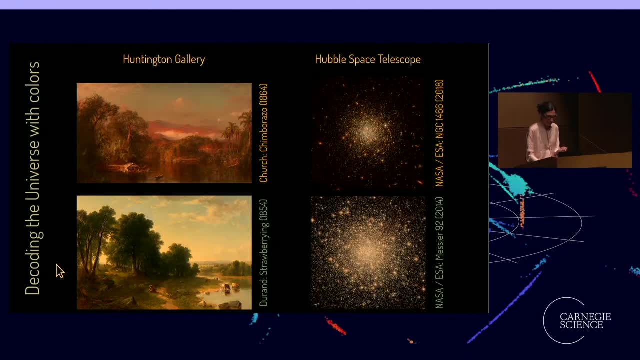 in true colors. The same is true in astronomy, although maybe not quite along the same lines. So here are two images of star, a global or clusters, imaged by the Hubble Space Telescope. On the top one is called NGC 1466,. 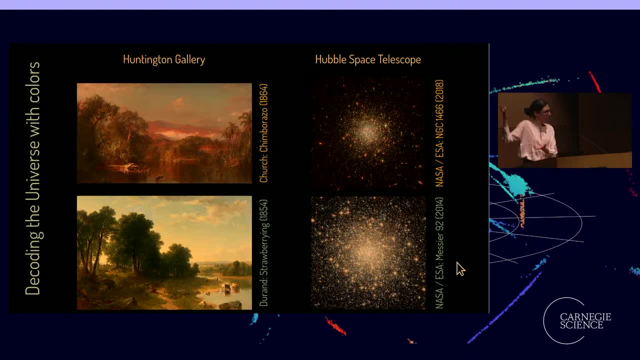 and the bottom one is Messier 92. They are both collections of million stars, 10 billion years old, and yet they look different. One is pretty red, the one on top, and the one on bottom is more blue. Anyone that's not an astronomer. 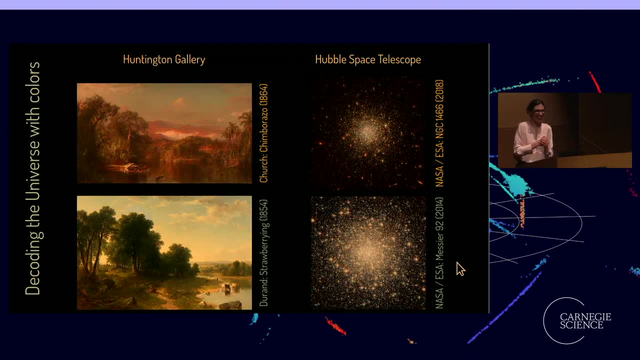 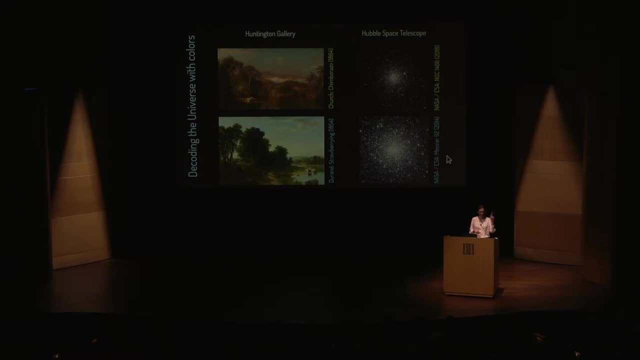 care to guess what the difference is? Older, Older, Very good. Warmer, Warmer Again. age temperature: The red one is collapsing. Ooh, the red one is collapsing. Okay, Dynamical state, That's dark matter. 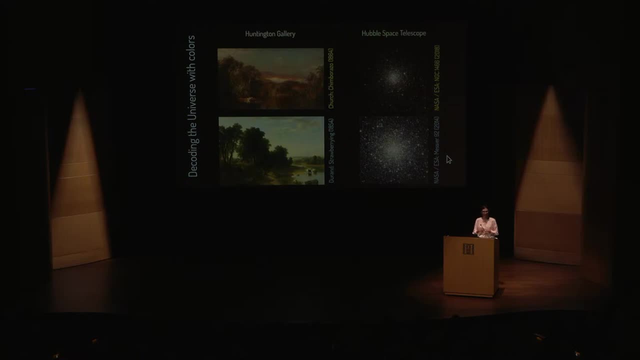 Ooh, dark matter, content, Interesting idea- Distance- Yeah, these are all great and definitely things that we kind of need to control for when we compare it once. but the aspect that will be interesting for us in this study is actually their chemical composition. 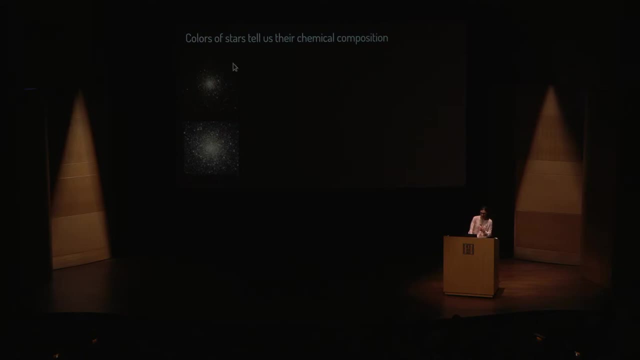 So when we kind of take light from one of these clusters and pass it through a prism, we get a spectrum like this. As you can see, that kind of underlying is like a nice rainbow, but then there are these kind of black lines. 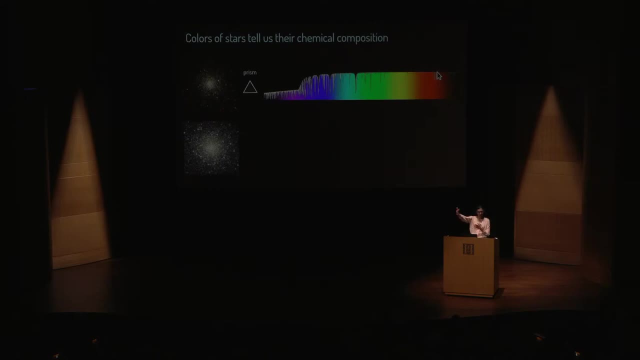 that mean that there is light being absorbed and not passing on through to us, And so for this one, you can see that there are some very deep lines. So these are hydrogen lines that are the broadest ones, but then there are some narrower ones. 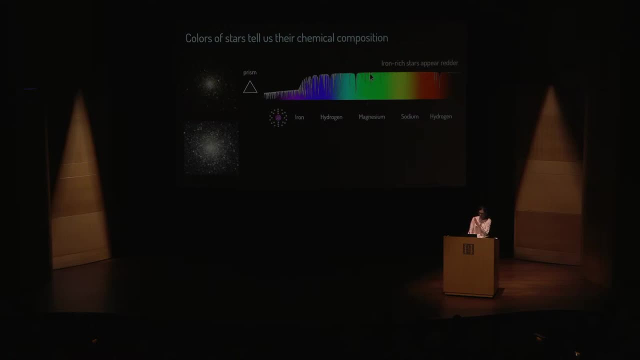 like the ones in the green part of the rainbow are from the magnesium, the ones in orange are from sodium, and then probably the rest of them, like there are other elements, but the safest bet is that they are actually iron, And so what happens is actually that light can get absorbed. 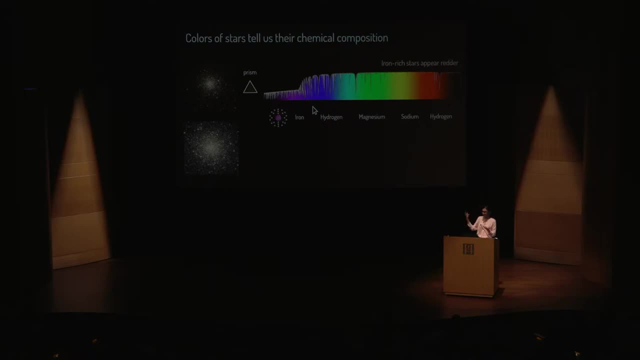 by the different chemical elements in the atmosphere, in the atmosphere of a star, and then that kind of color of light gets diminished. And iron is really good at blocking a lot of lights because it a lot of light, because it has a lot of electrons. 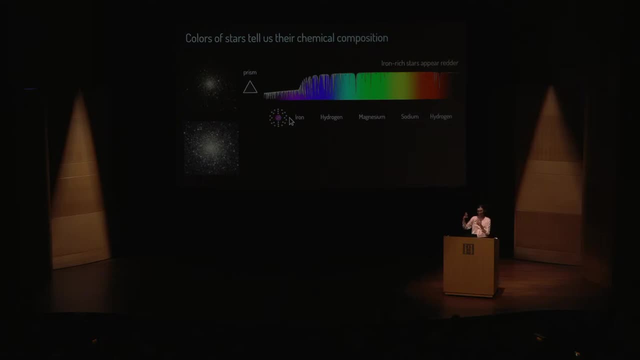 So it has 26 electrons and so they can all observe like various different colors of light and light of different energies, which means, and as you can see, there are a lot of these lines in the violet and blue and kind of. 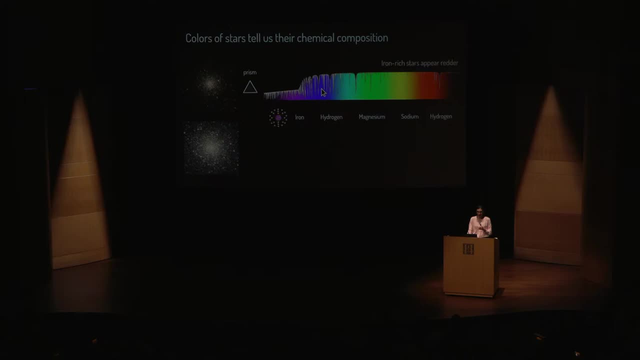 the teal part of the spectrum over here. So it means that on average, if there is a lot of iron on a star, it will appear redder. If we take the spectrum of the bottom cluster, which is more blue, we see that there are still some of these same lines. 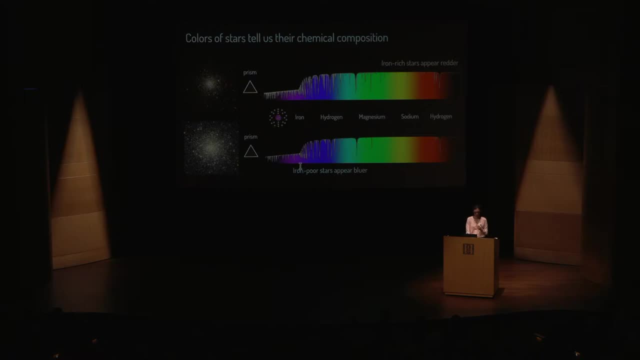 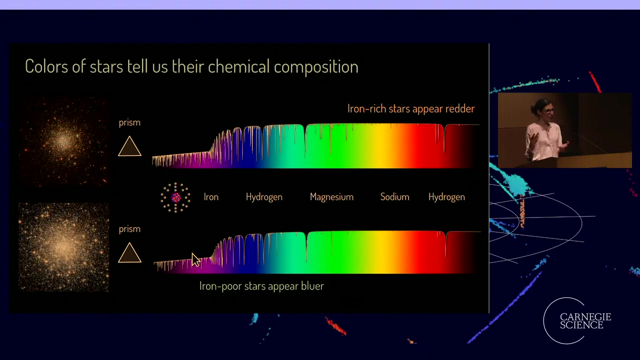 they're all a little bit weaker and there's much fewer of these thin iron lines. So that means that on average, the star that has less iron will appear bluer, And so this will become- or really became- kind of a standard tool. 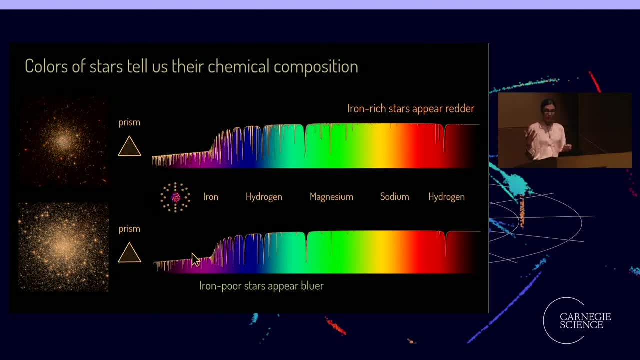 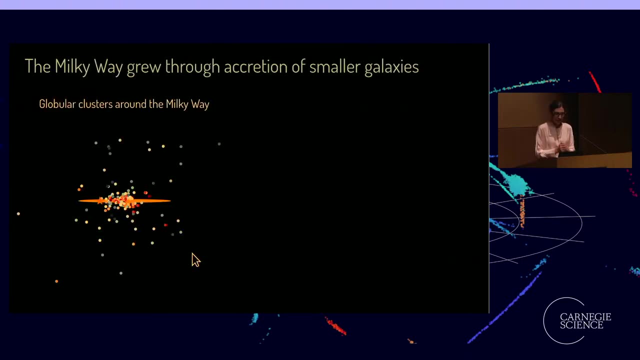 for understanding the origins of different structures in the well different stars and also different structures in the Milky Way galaxy. So I'll here introduce a study that was done by Leonard Searle and Bob Zinn, who were also Carnegie astronomers, back in 1978. 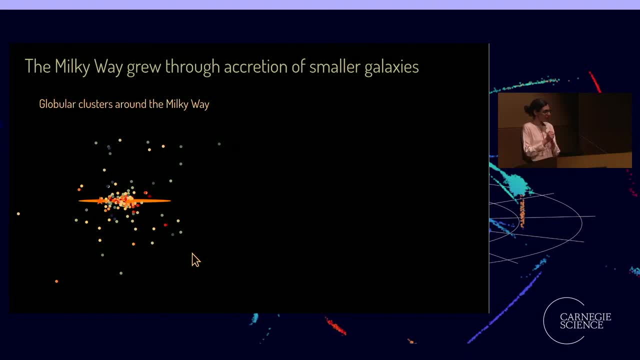 And so what they were studying were groups of these clusters that are spread all around the Milky Way galaxy. So as a cartoon I'm showing here the structure of our galaxy, kind of viewed edge on where the sun is, here in this disc. 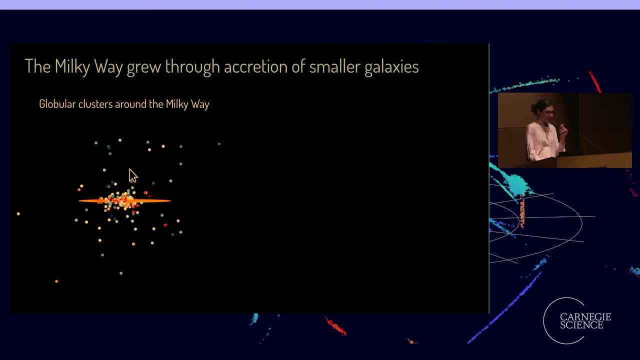 and this is the center, so sun is a little bit offset, and then the points are the well currently known globular clusters And the color kind of corresponds to the actual color. As you can see, there are a lot of kind of blue ones on the outskirts. 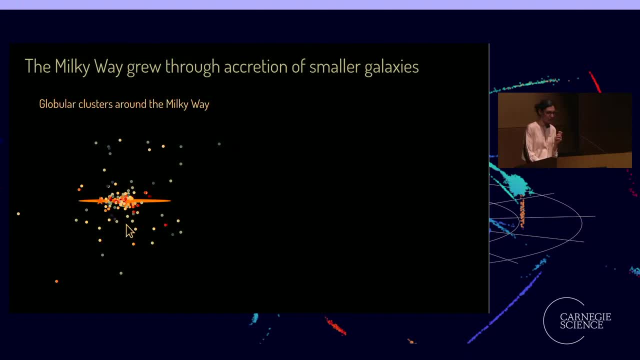 and more redder and orange ones close to the center, And so this is basically what Searle and Zinn did was to quantify this measurement. So this is a graph directly from their paper showing the iron abundance on the y-axis. 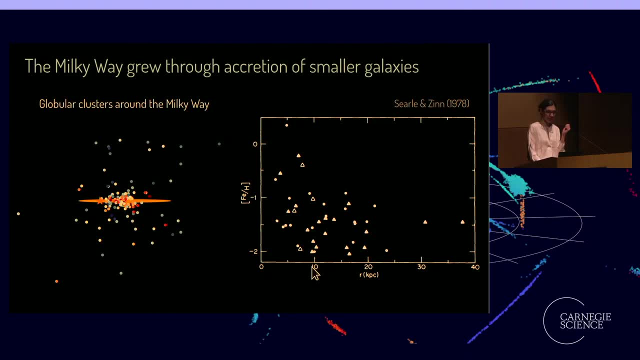 and then the distance from the galactic center on the x-axis. We today know of more than 150 globular clusters. They only had measurements for 19 of them Because it was painstaking work even then, But what they found was something very foundational. 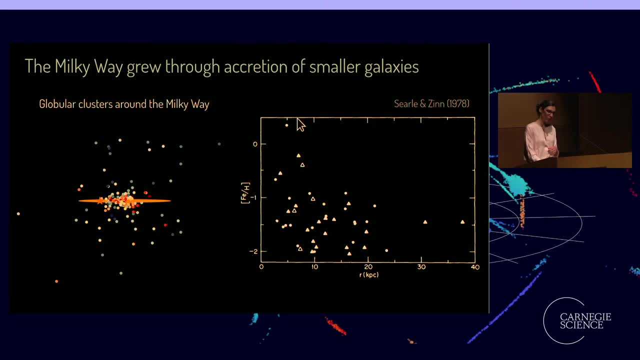 So what they noticed is that for some of these most clusters closest to the center of the Milky Way, they can have, they have a ladder of iron And then, as they were moving away from the Milky Way center, it kind of the iron abundance dropped. 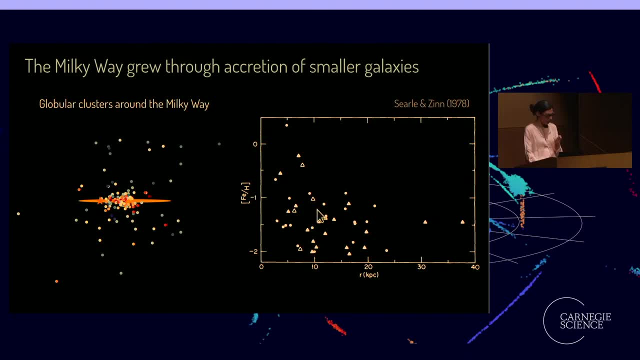 Until they kind of came to the distance of the sun, which is around eight kiloparsecs, And then they found that the iron abundance dropped. And then they kind of the iron abundance dropped, And then they found that the iron abundance dropped. 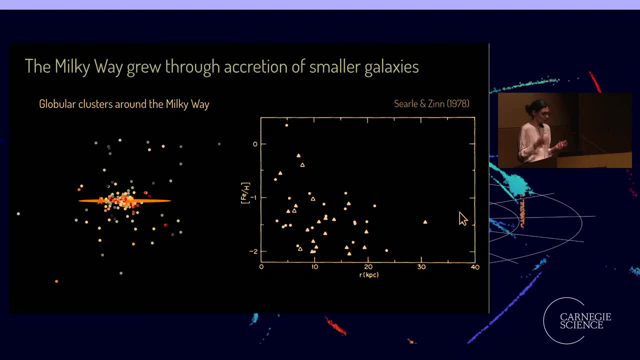 It kind of stayed flat all throughout, And so their expectation was okay. if there's like a lot of stars being born and generating a lot of chemical elements, they can kind of pass them on to next generations of stars, so they should be kind of getting a lot of iron. 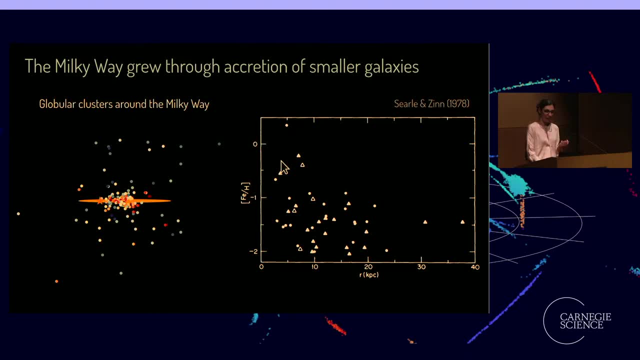 And that was kind of what was happening at the center of the Milky Way, And then they expected, like this would just continue to fall off, because it will be just like most of the stars will be at the center of the Milky Way. 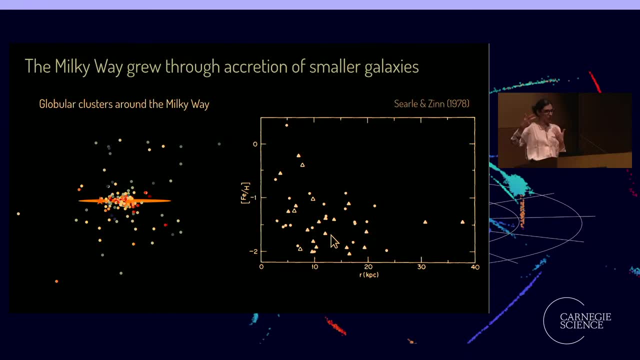 and then will be kind of less and less and less kind of contamination with iron and other elements. But what was surprising is that it actually kind of didn't continue dropping off, but it actually stayed pretty constant. And what they concluded is that indeed many of those clusters didn't really form in the Milky Way. 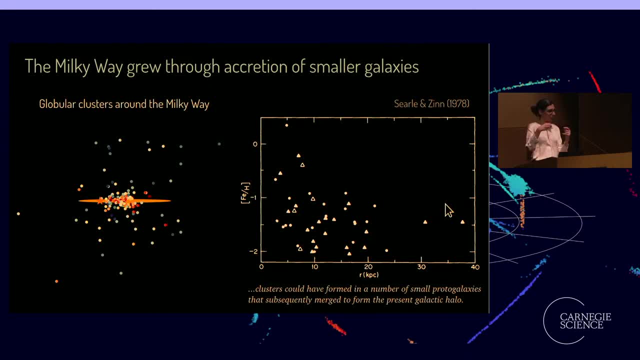 but formed in other smaller galaxies that were then later brought onto the Milky Way, And what they actually says, or how they called it, that they could have formed in a number of small proto-galaxies that subsequently merged to form the present galactic halo. 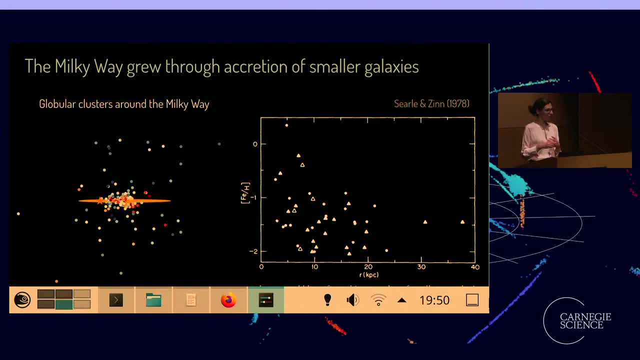 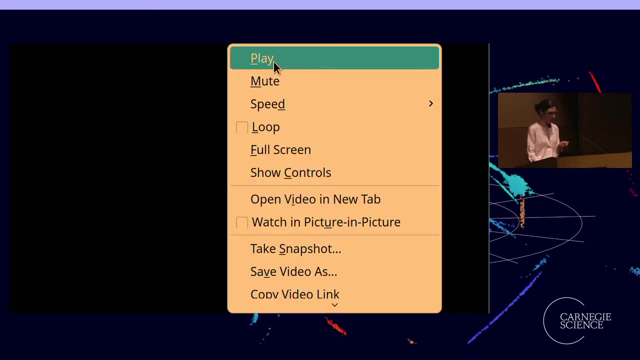 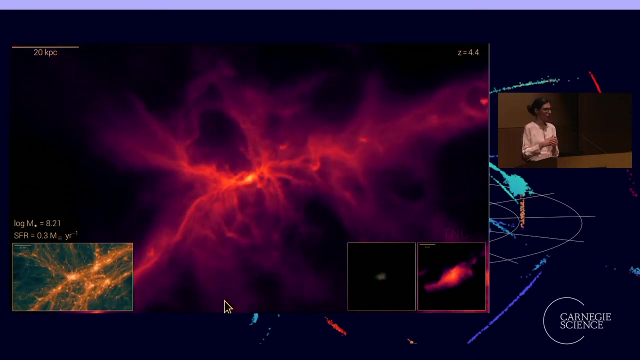 So this was kind of similar to what we expected from those very early simulations that have 700 particles and said that galaxies should be growing by merging with each other. Today we have much more advanced simulations. So here play a movie From the illustrious TNG project, which is a large collaboration centered in Europe. 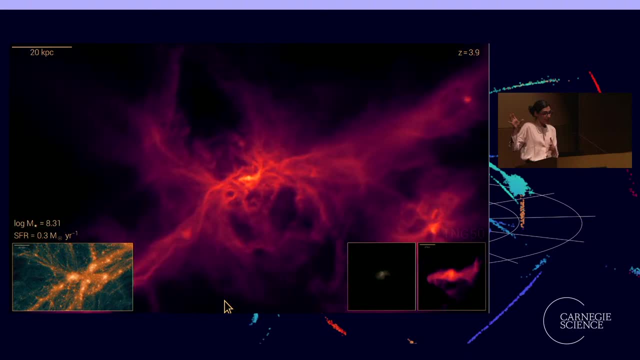 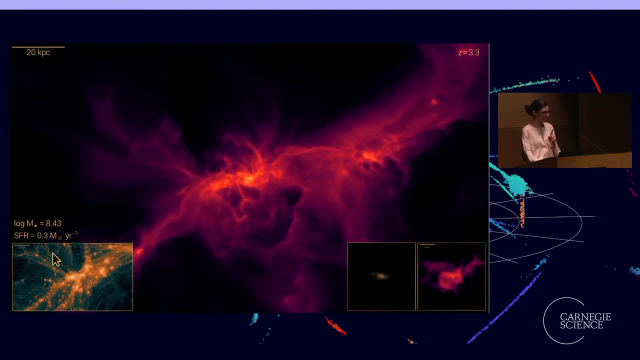 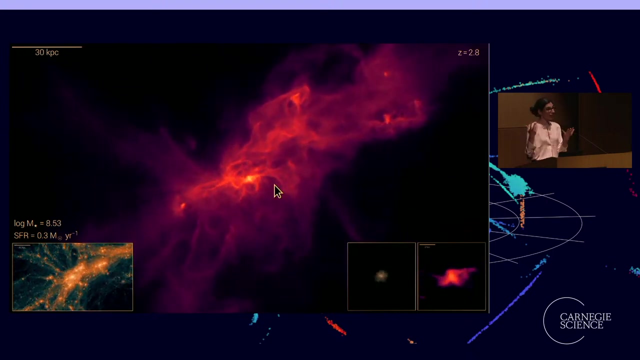 And this is one of their Milky Way-like galaxies seen in forming. So the dark matter particles they have, 2 million of them are shown here in the bottom left. What we are seeing here on top or on the center is the gas particles. 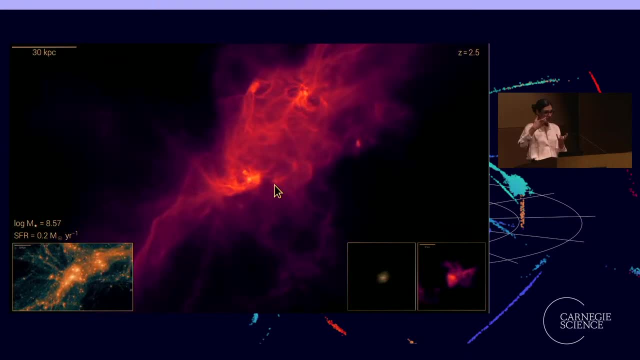 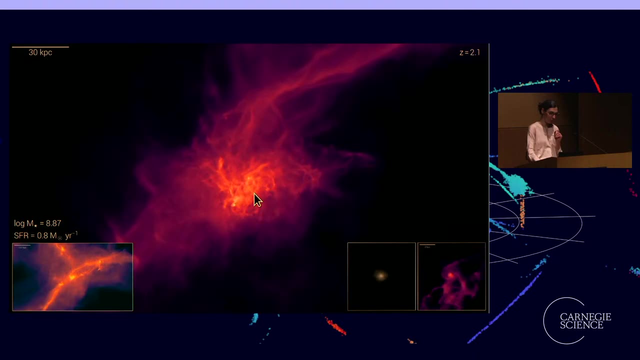 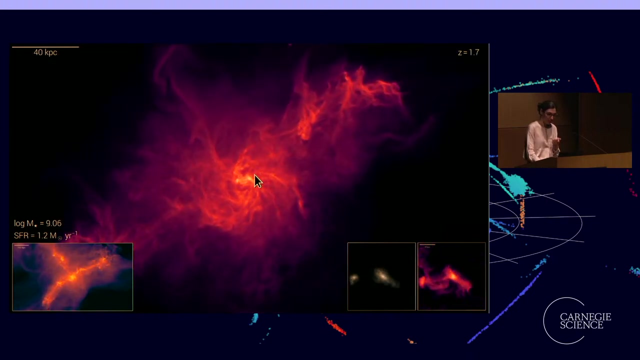 So they're not really only tracking dark matter, but also kind of gas. So you can see that there are now two objects merging to each other to form a more massive one, And what happens in this very densest regions of the gas is that it actually starts forming stars. 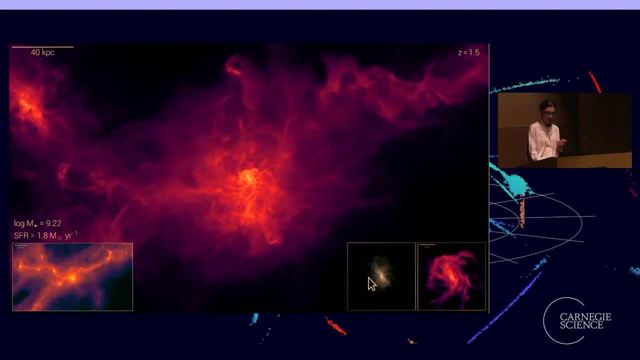 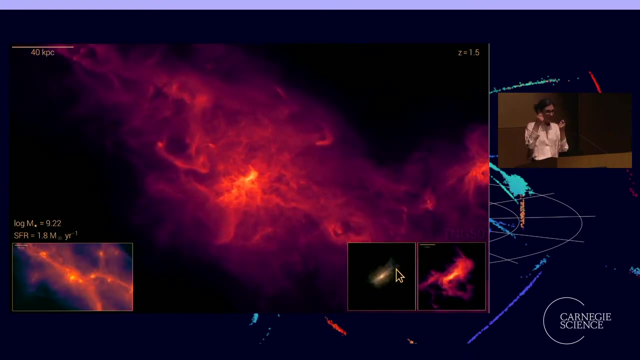 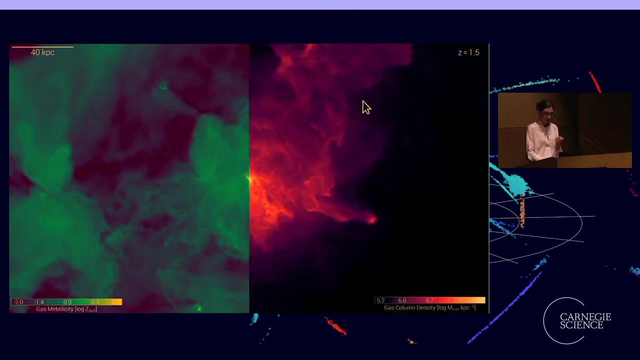 So the stars forming are shown here in the bottom inset. So now we will see just kind of how high of a resolution this is and how intricate these filaments are. And we are also seeing them in density on the right and then in the metal abundance. 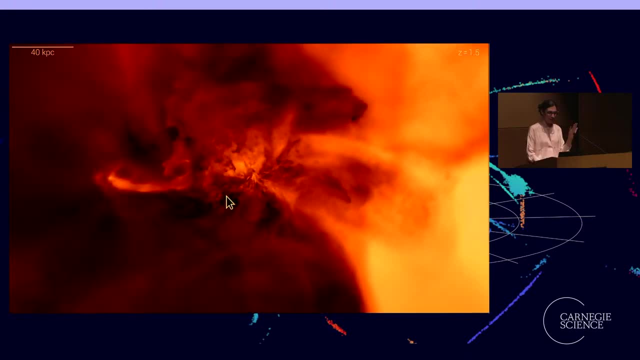 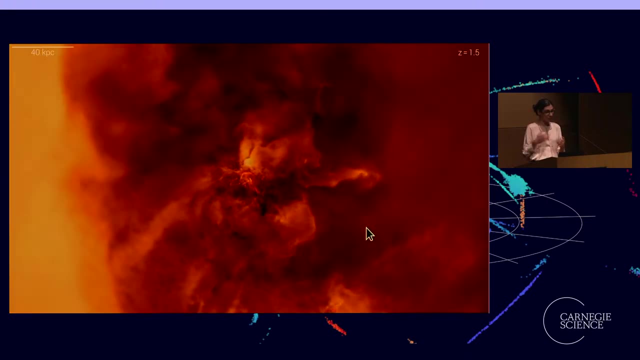 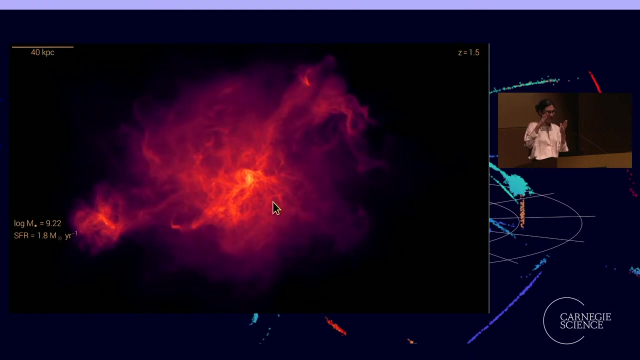 or rather abundance of iron elements on the left. Now they are showing how fast this gas is moving. So these are all properties that are being tracked in this simulation, And this is now kind of what will be unobservable if we were able to observe a galaxy at different times. 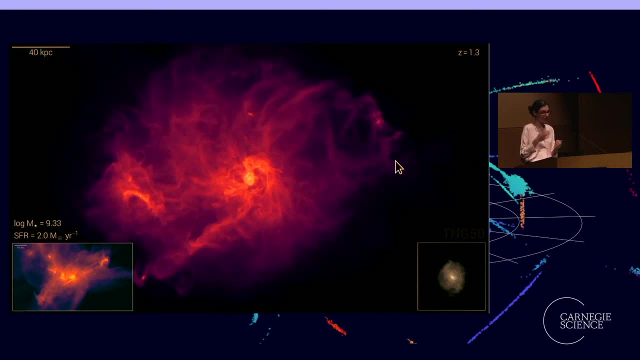 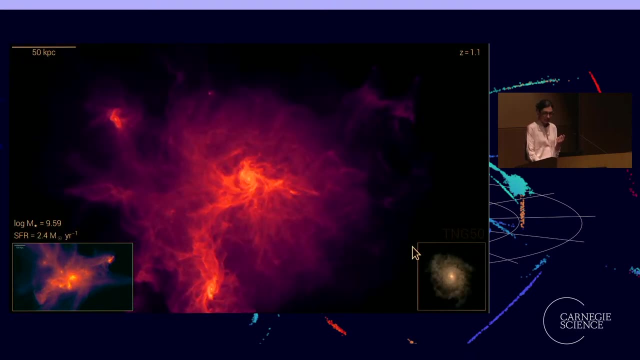 So this is something like 6 billion years old And this is something that we have seen in the past, And now we are kind of continuing to move on, still seeing the gas in the center and then the spiral galaxy forming the stars on the bottom right. 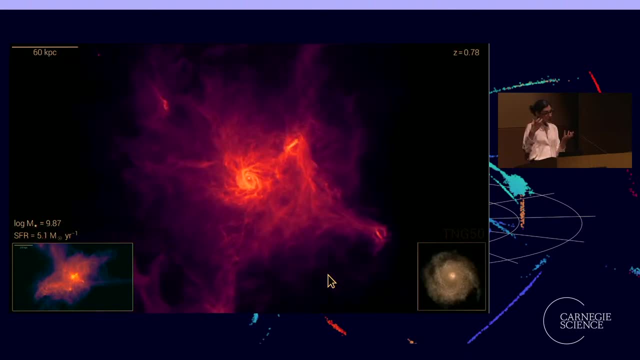 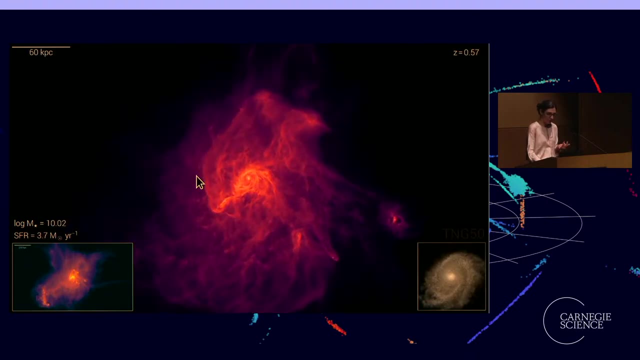 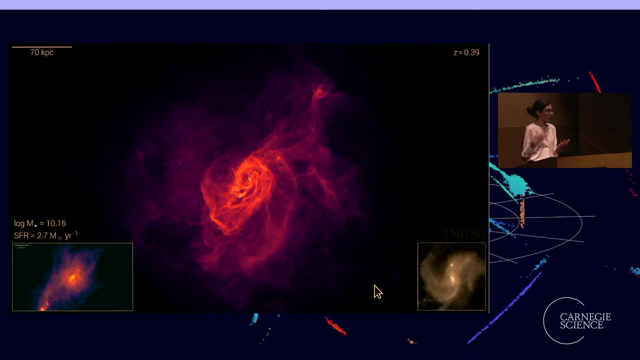 As you can see, now, this process of merging continues on and there are small galaxies that are coming in, kind of being transformed into these huge ribbons of gas and also stars, to finally form something that really looks like a, a spiral galaxy that we think our own Milky Way is. 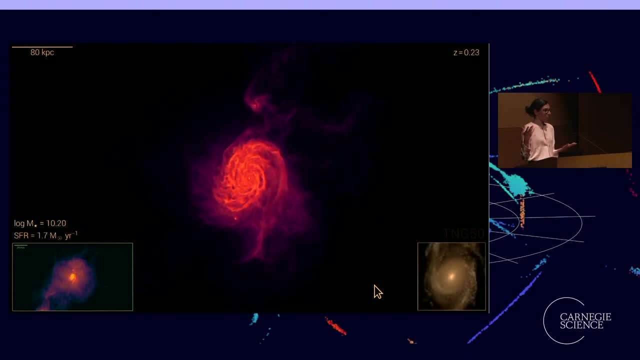 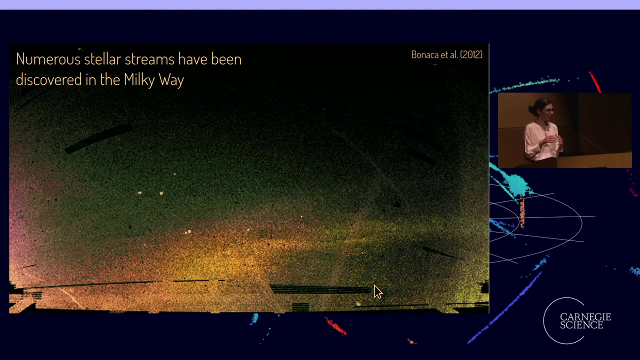 And so this now kind of paints a more complete picture of how we think a galaxy like the Milky Way was born. What we kind of wanted to do next is actually test this. Do we actually see this merging in progress? And so we kind of learned from Serlin Zinn. 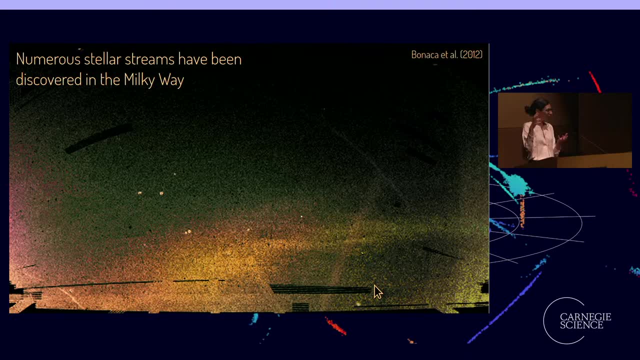 that the outer parts of the Milky Way have clusters that are typically bluer. So once we imaged large areas of the sky, we actually went to look for blue stars, And this is how I, or how my own journey into astronomy started. 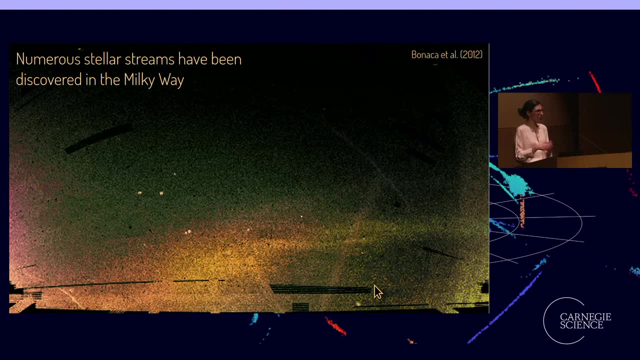 It was when I walked into my future advisor's office for my PhD And she said like, oh, it would be great if you kind of looked at this new data set from the Sloan Digital Sky Survey and just look for some of these blue stars in the halo of the Milky Way. 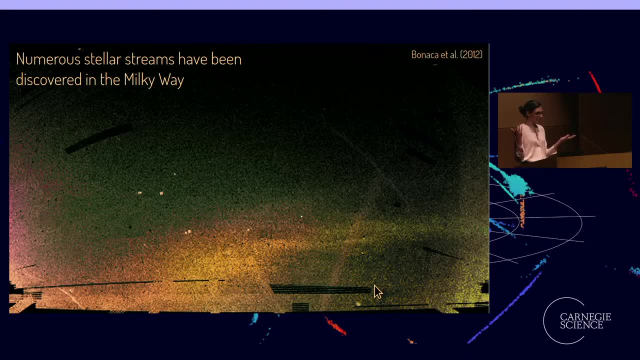 and see if there are any structures. And turned out they were and lots of them. So this is one of the images that I created as my very first year project. So this is a map of the distant structure in the Milky Way halo. 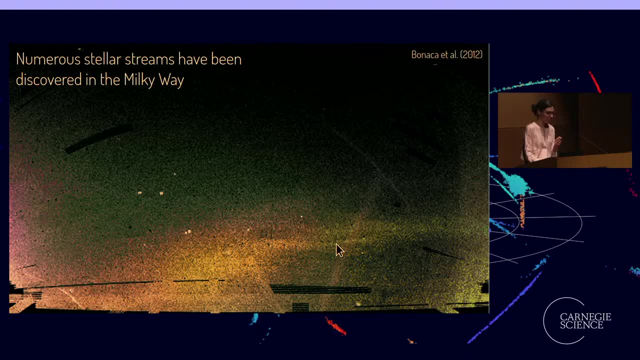 And the different colors are mapped to different distances, And so the most obvious kind of clumpy things are like these bright dots. So these are. many of them are globular clusters, some are small dwarf galaxies, But then you can also see some of these very kind of 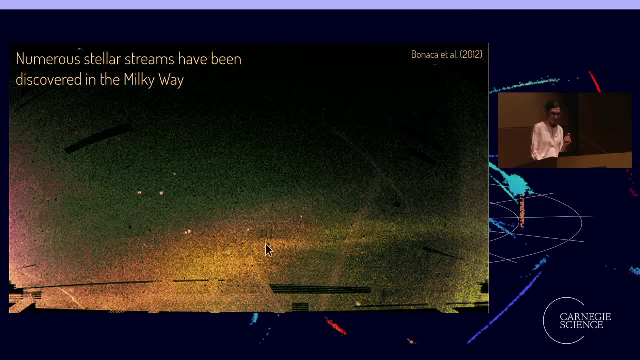 streamy regions of the of the plot, And so we think those are sort of dwarf galaxies in globular cluster, globular clusters that are in the stage of being kind of merged with the Milky Way, So the longest one over here is called the Sagittarius stream. 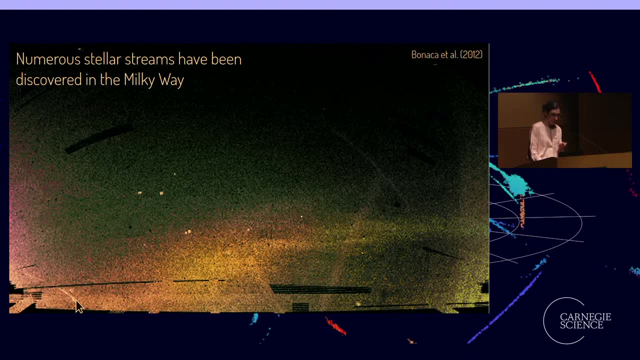 The thin one over here in the bottom is actually the Palomar 5 stream, So the cluster itself is visible just as a tiny bright dot, but then it has, like these huge extensions of kind of tidal tails around it, And so this was super exciting because, yet again, 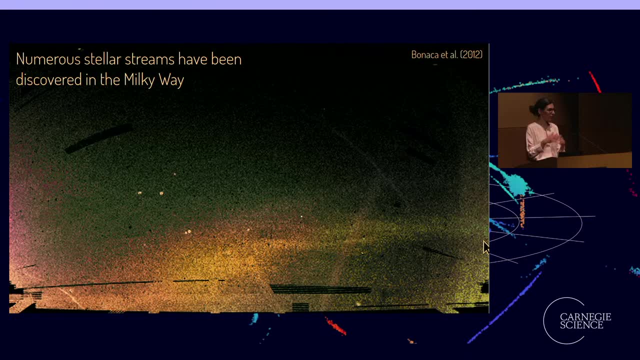 it was another confirmation that this basic picture works. So the simulations predicted there should be objects kind of currently being brought onto the Milky Way and depositing in their their stars under our own galaxy. And then we were able to find them with the, with the observational data. 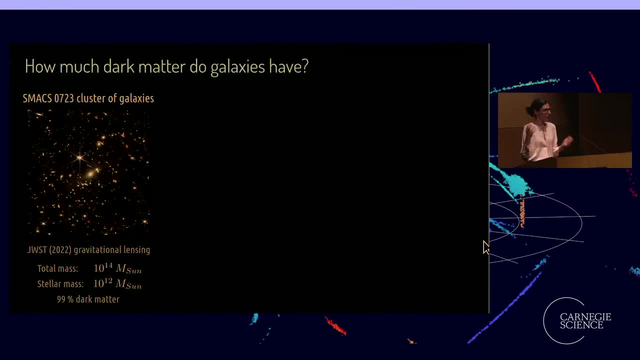 And then the question was: okay, so it seems like this model of the universe, where really there is like a lot of dark matter, seems to be working well. And then the question was: exactly how much dark matter is in the universe? And so this is still a very 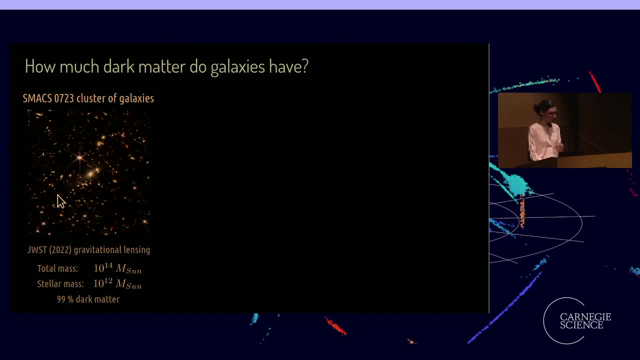 very active question and perhaps you've seen an image like this. This is JWST, the new space telescope view of the cluster of galaxies that is being. that is lensing galaxies that are behind it, And so, because of this lensing- gravitational lensing- 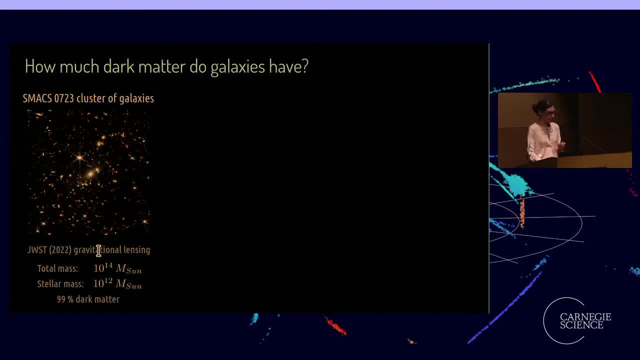 astronomers were able to calculate what is the total mass of this cluster of galaxies and then find that it is 100 trillion solar masses, Whereas if they just counted up the mass in the galaxies themselves, they found that it's only 1 trillion. No, 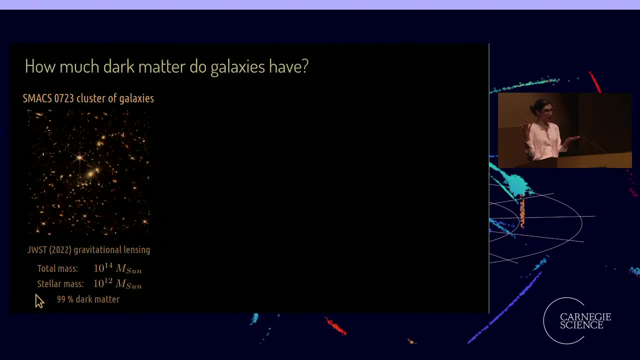 But that means that, like 99% of all of the matter is dark or invisible. So in the Andromeda Galaxy we're already familiar, but I thought I would include it here because it's a very different mass scale. So we see something that is very massive. It's like 10 to the 14 solar masses. So the mass of the Andromeda Galaxy and the Milky Way is pretty much the same. The total mass is 1 trillion solar masses, And then the stellar mass is 100 billion solar masses. 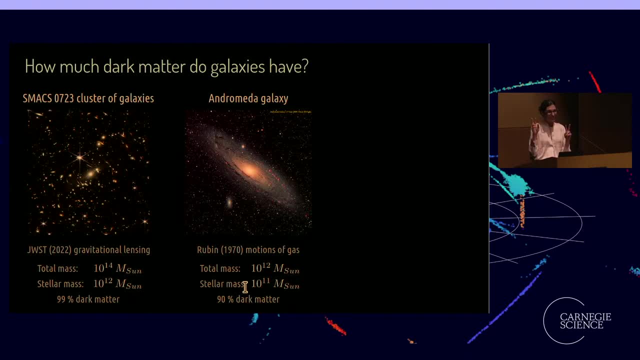 So, which means that, okay, this is only 90% dark matter. Then we have even lower mass galaxies, like one that orbits the Milky Way galaxy, And this is one of the most recent discoveries, called Reticulum 2.. It is so faint. 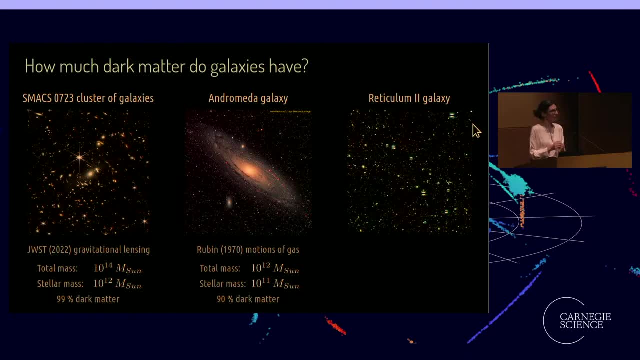 Even if the room was darker, it would be really hard to see it. But there is a slight over-density of bluish stars here at the center, And then the question is: what is the dark matter fraction in this galaxy? If you had to guess, what would you say? 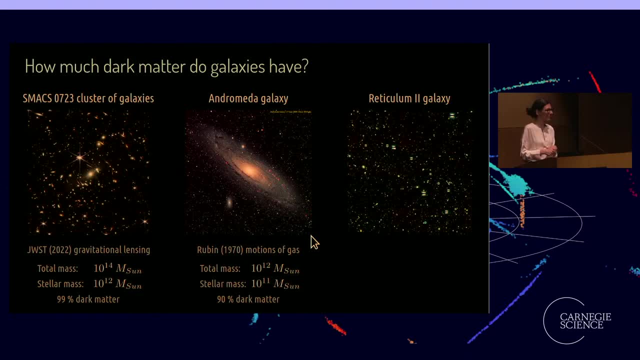 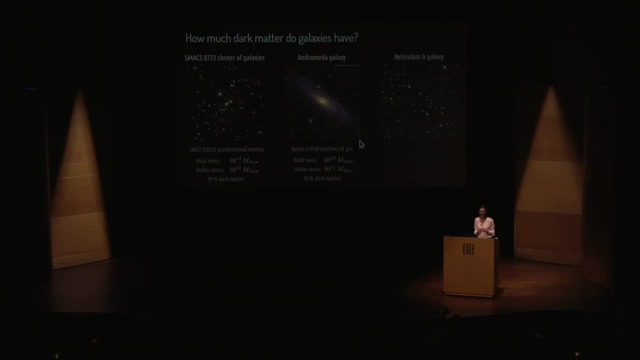 Fifteen, Fifteen, Eighty, Eighty, Thirty, Thirty- Wow, You're really covering our bases. Anyone for over 90?? Yes, Yes. Anyone for over 99%? Yes, Yes, Some, yes, Okay. 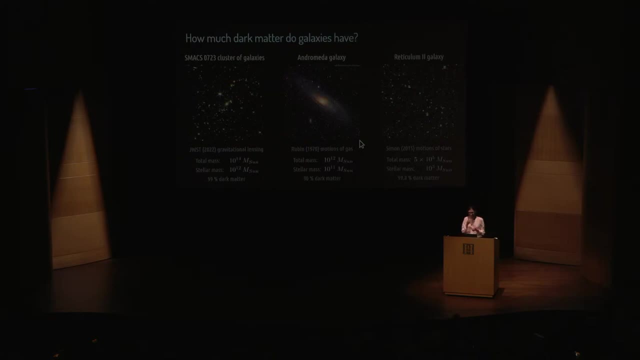 It's 99.8.. So this is one of the most dark matter-dominated objects That we know of. And then the question is: okay, it looks like there are, like, if we go to, kind of these smaller clumps, so you see, like the total mass is much smaller than that of the Milky Way. 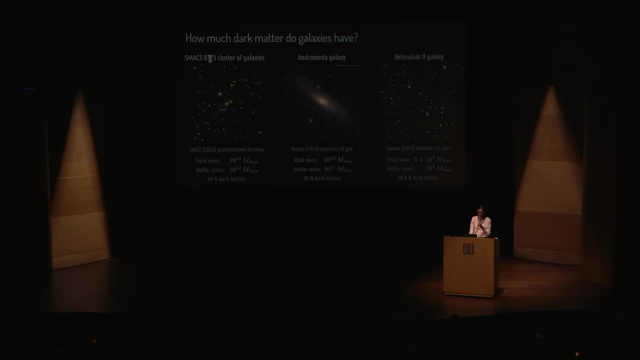 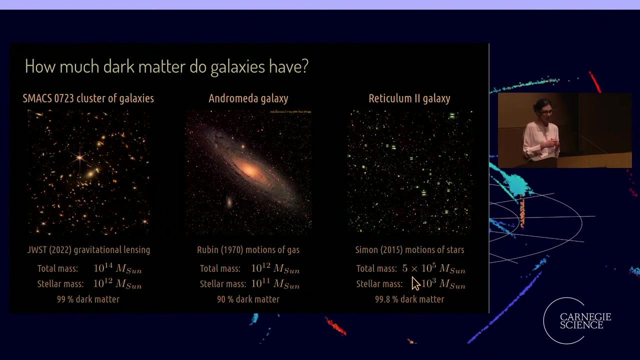 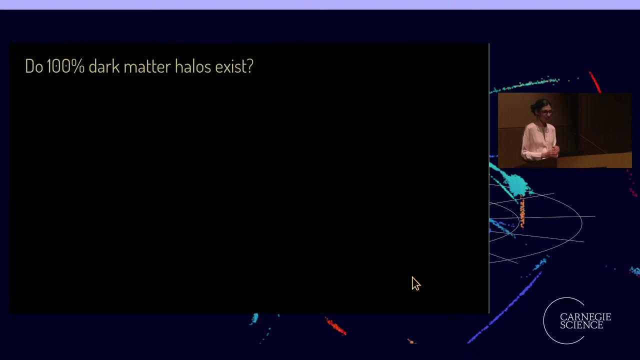 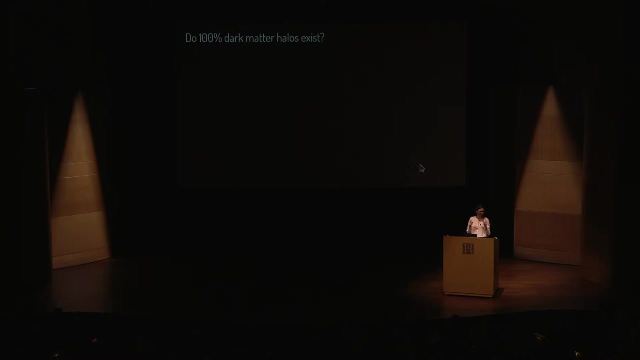 or of this SMACS cluster. It's only half a million solar masses. Then the question is: do objects exist that are 100% dark matter? Yeah, who thinks yes, Show hands? Yes. Who thinks no? Okay, There are some brave people who are. 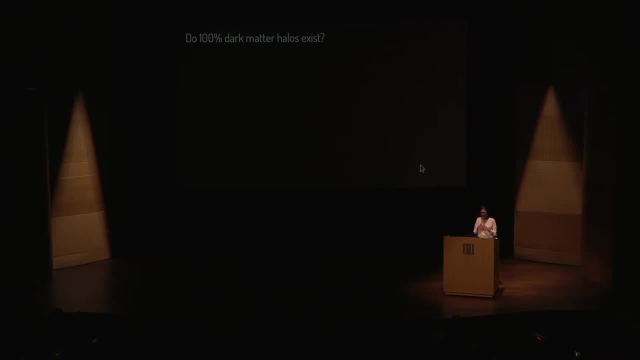 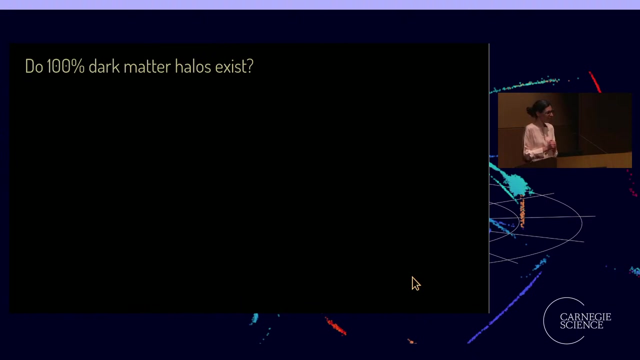 I know I kept saying like we have, like you know, more than 90% dark matter. But this, the question that we don't know the answer to, And I really want to find out, because you could all be right. 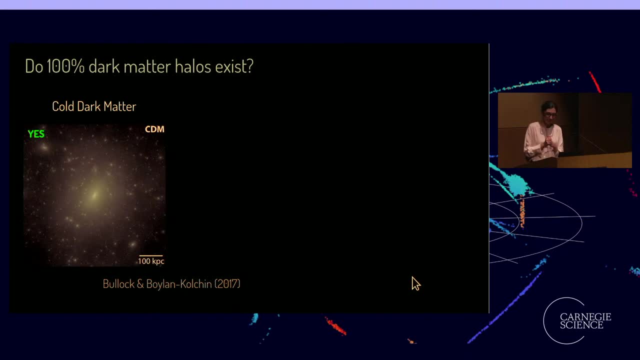 So in our standard model of cosmology, we think the answer should be yes. A galaxy like the Milky Way has this massive halo of dark matter which is full of smaller clumps that we call subhalos, But this is just one model of the universe. 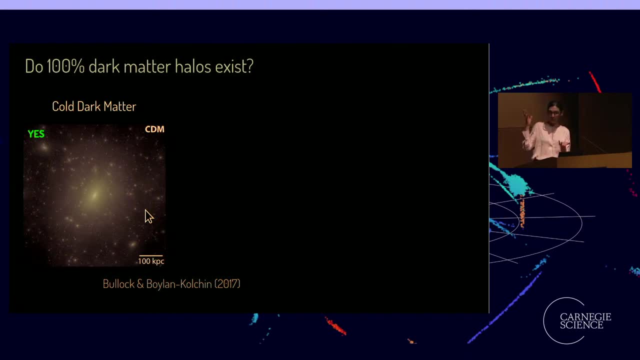 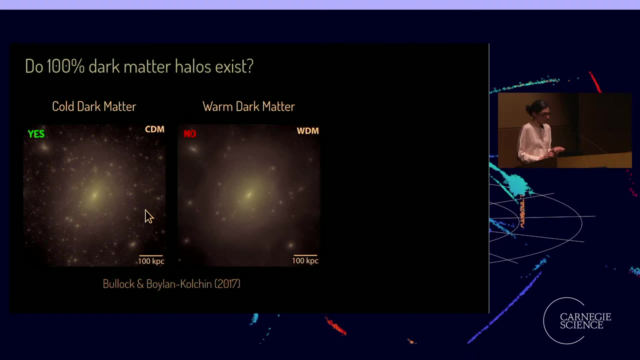 and cold dark matter. in this case is a massive, pretty massive particle which we haven't seen in the lab, so it's still hypothetical and they will not exist. The particle could be lighter and that would mean that all of these smaller clumps are kind of too light. and the particles are moving fast and they can just kind of go away. And if dark matter is warm, then the answer is no, that there actually shouldn't be any clumps of dark matter that are only dark matter. There are different kinds of models. 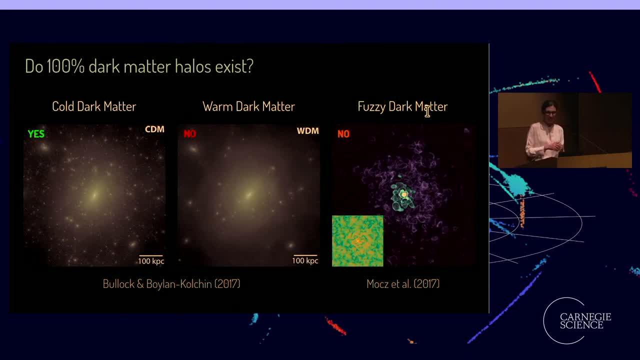 called fuzzy dark matter In this case, where the dark matter is such a super light particle that the kind of quantum interference effects are seen on these macroscopic scales, scales of galaxies. I put no in orange just to distinguish it a little bit from the red one, because 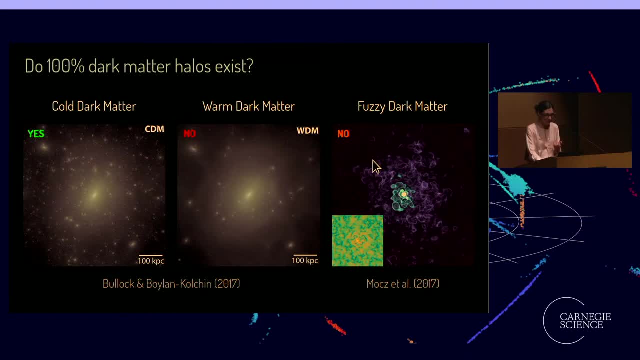 while there are no kind of bound clumps like there are still, you know, see these intersections where kind of waves are crossing, that could be kind of pretty low mass, but only for a little while, and then kind of dissolve. 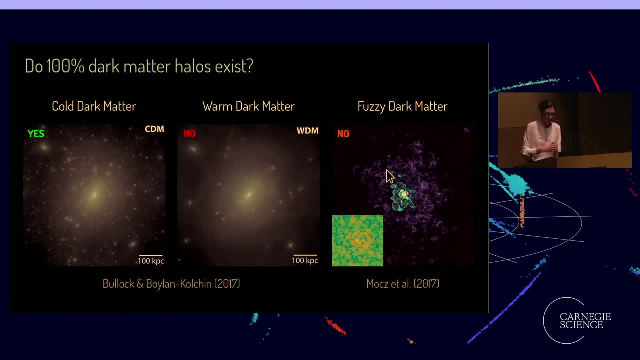 So it's some even more unusual type of dark matter than the other ones which we have studied so far. But this remains the main question of my own work: Do 100% dark matter, halos and subhalos exist? And so the question is: how do we tell? 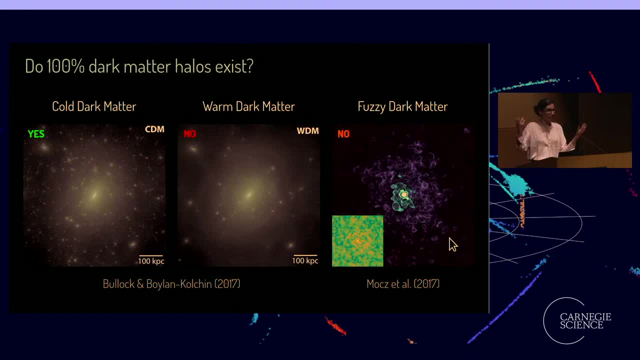 They are invisible. We said we can measure that there is dark matter from its, the motions of the stars in the Milky Way, but like this should be like a million times less massive. so the effect would be pretty small when they were interacting with any individual star. 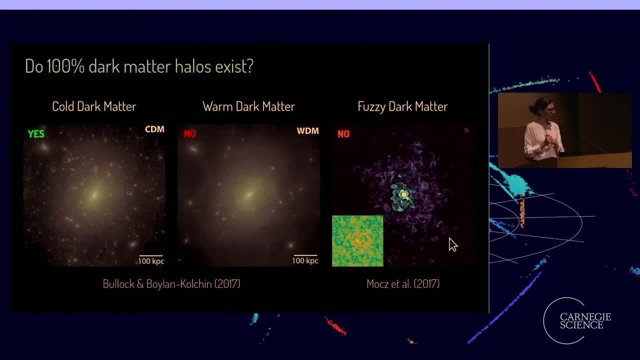 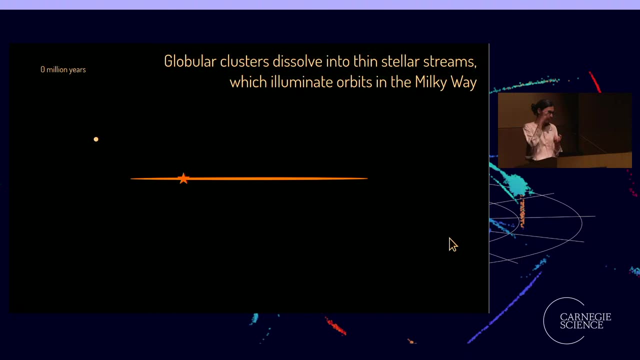 But turns out that our friends from before the globular clusters come in handy once again. It turns out these when they move around the Milky Way. okay, I'll play this movie. what happens is that the gravitational forces of the Milky Way 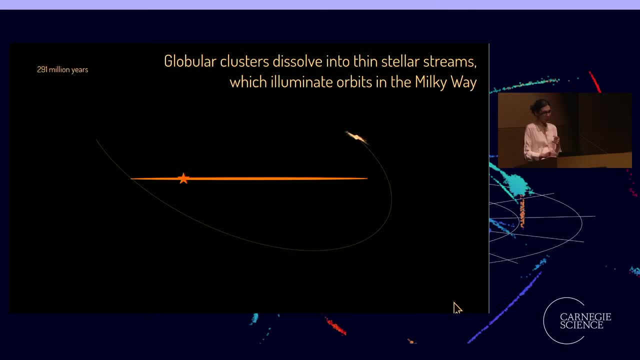 start pulling stars out from the cluster And kind of little by little. so the timer is here well, going pretty fast, but not super fast for astronomical terms. over millions of years, kind of. the cluster loses its stars And they kind of form this very thin stellar stream. 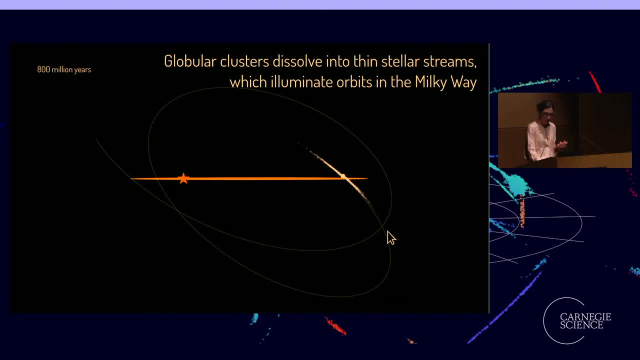 And for the most part you can see, it's kind of aligned with the orbit of the cluster. So that means for this, this particular set of stars, we kind of know where they should be Like if there is no dark matter clumps. 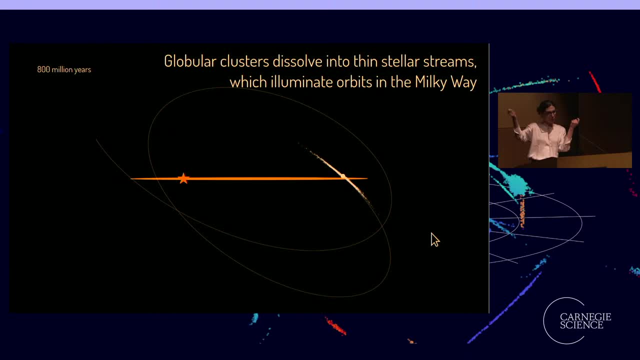 they should be kind of following this like pretty regular kind of one-dimensional. I can imagine it just like as a string somewhere in space orbiting the Milky Way, And this is important because the situation looks pretty different if there is a dark matter substructure. 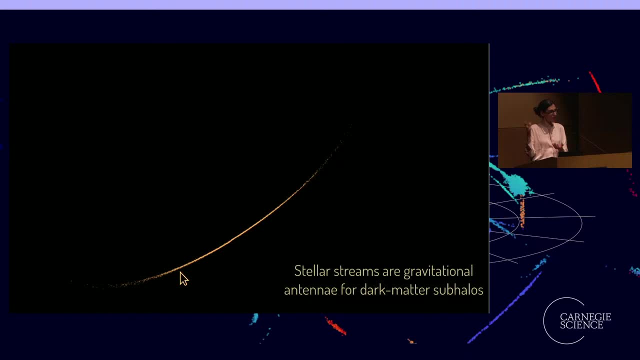 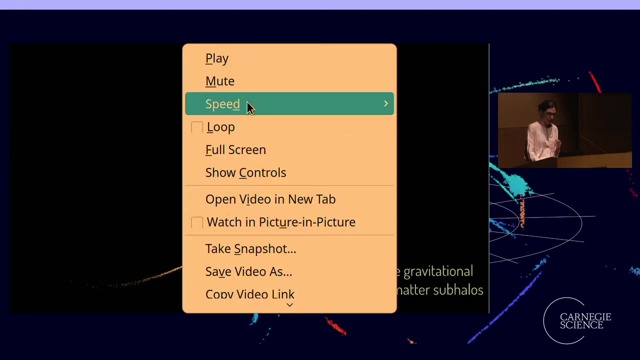 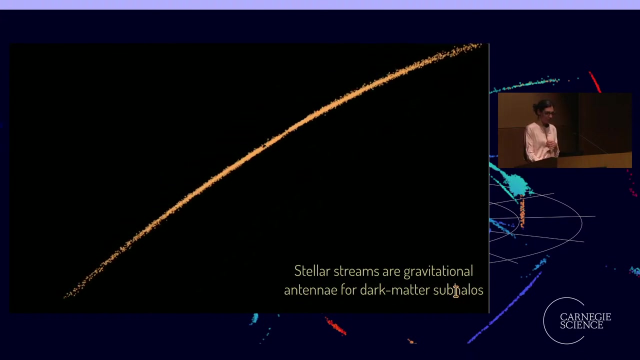 or a dark clumps of dark matter. So this is basically the same stream, just from like a few, like a billion years earlier and seen from a different angle. It's kind of moving on its own until it encounters a massive object. 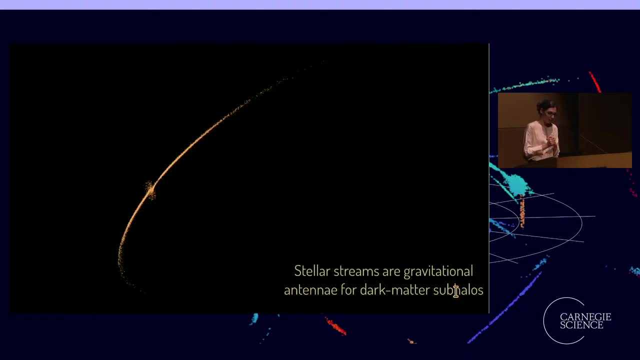 It kind of passes through the stream and gives kind of a velocity kick, kind of kick stars out of the stream And so they are no longer moving as we would expect them to be, all kind of one after the other, but they're kind of puffed up. 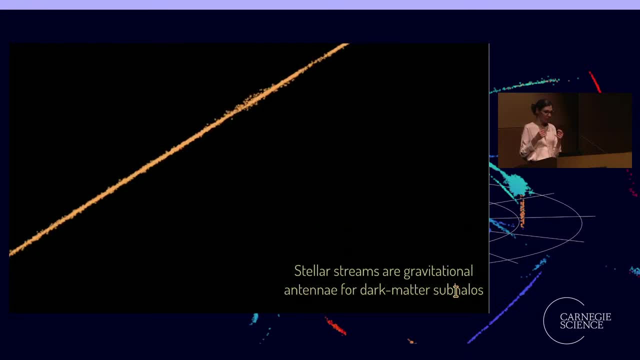 around their original orbit. And when we look at them today, what we see is this structure that has some stream stars kind of out of the main part of the stream and where they used to be there is a small under density or a gap. 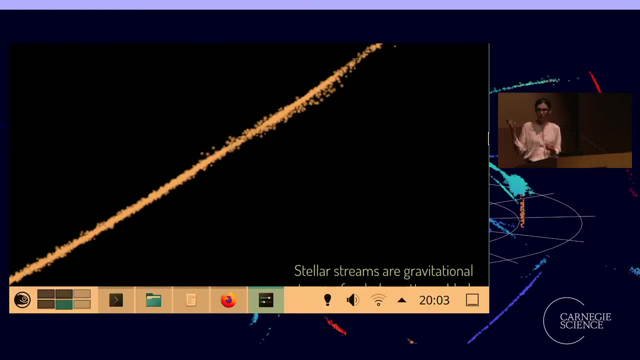 And so this is one way- and turns out one of the most precise ways- with which we can determine whether there are clumps of dark matter that we otherwise wouldn't be able to see. So again, theory was like: okay, very super clear cuts. 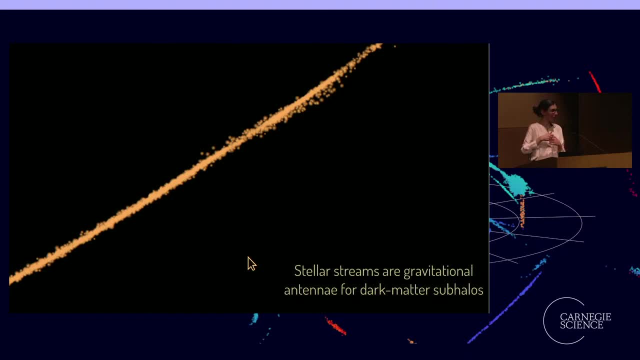 like should just go observe, like go back to your map of stellar streams in the Milky Way and check if you see such structures, if there are like some stars kind of outside of the stream and if there are like some variations in density along the stream. 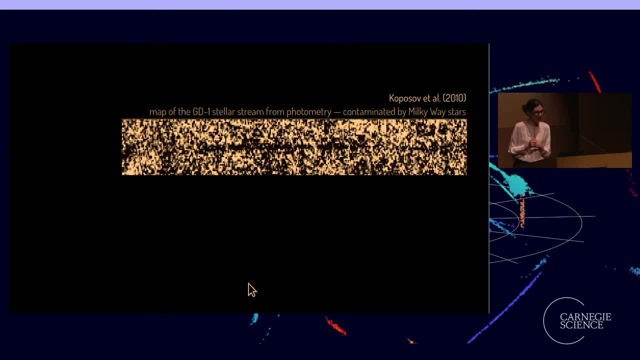 The issue is that data was actually pretty hard and a different story. So this is. this is showing a map of one of the stellar streams, one of the most famous stellar streams known in the Milky Way called the GD1. And this map is pretty similar. 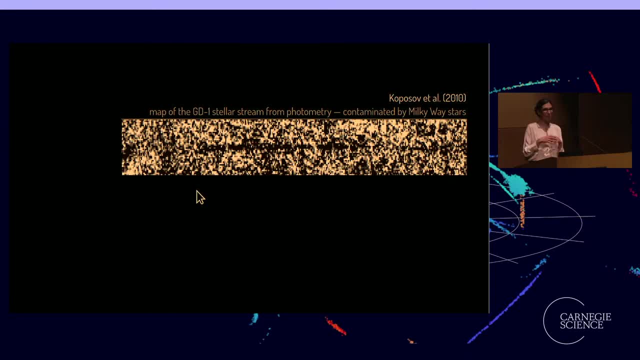 to the one that I showed you before, which is again basically measuring the density of bluish stars of a particular brightness, And so you can definitely see, I should say, these are sky coordinates, So just kind of oriented in such a way. 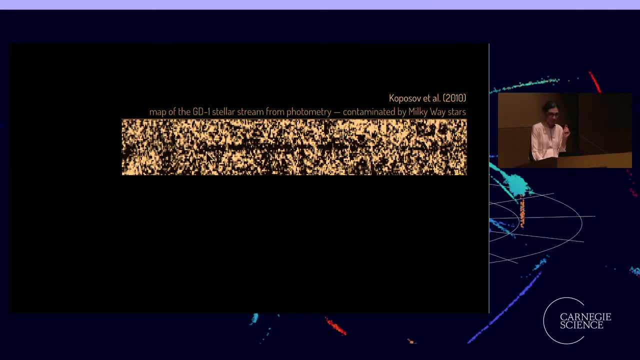 that the stream is passing through the middle And so the darker means higher density. So you can definitely see that there is like this black stripe through the middle of where the stream is. But then if you were pressed to say: are there variations in density along this line? 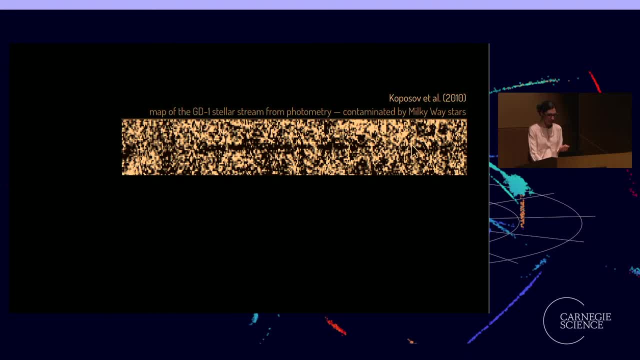 It's kind of hard because you might say like: oh, maybe there's like an under density here and over density here and under density here, But then if you look kind of above or below the stream, you can see similar variations in density. 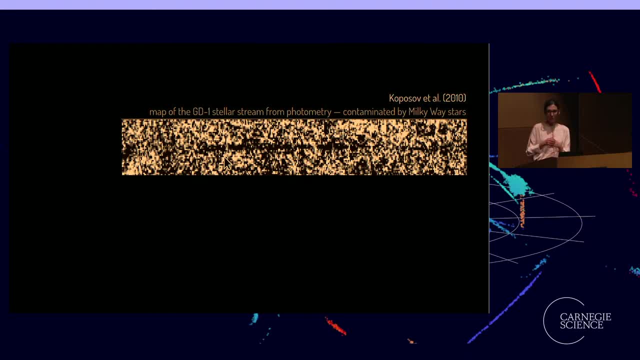 which means that it could be actually very well the variations in the stars, the kind of that, are other Milky Way stars not part of that stream structure that are contaminating our view, And so this was the case for some time. So this is a work from 2010,. 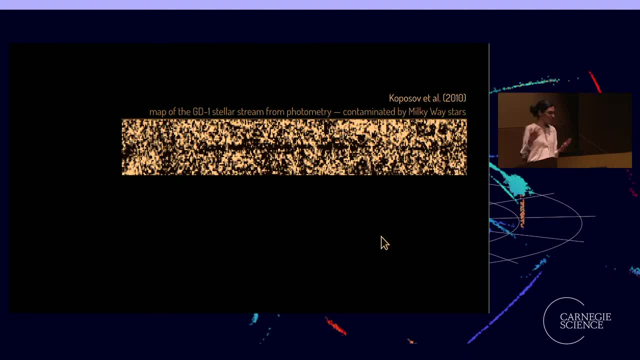 but then we were really fortunate in this field of sort of galactic archeology where we're kind of trying to unearth what happened to stars in the Milky Way. So we were really fortunate that European Space Agency mission Gaia flew And what Gaia measured were velocities of stars. 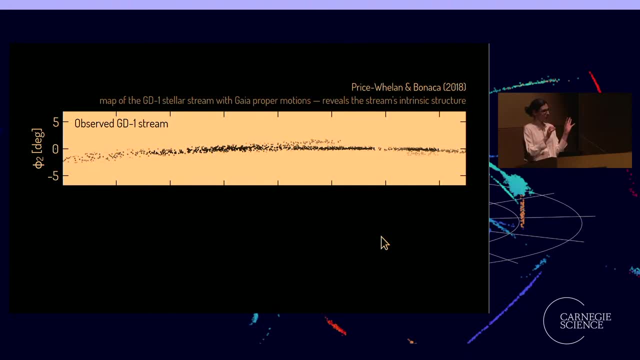 And so what we were able to do is then select only stars that are moving in the same direction and get a map that looks like this. So this is a super clean view to what we had before, And this was in 2018, when my collaborator 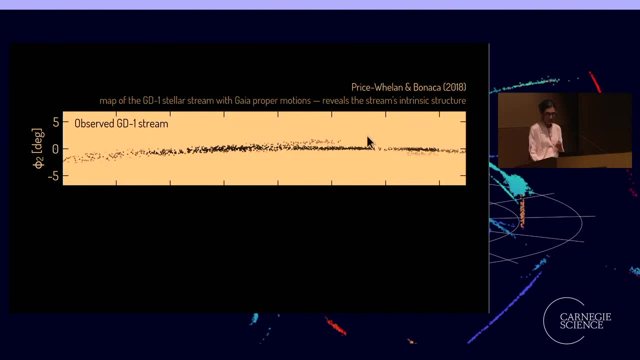 Adrian Price-Wellen and I measured really precisely the structure of the GD1 stellar stream And we found that there indeed are density variations. There is one gap here that is very prominent, There's another one less prominent over here, And there are even hints of these stars. 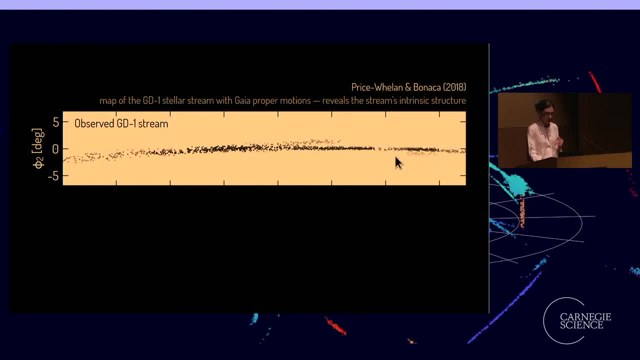 that are kind of flung out of the stream here on top and on bottom over here, And so this was the data was so fantastic that really creating this figure took maybe three days, And then we spent the rest four days writing up the paper. 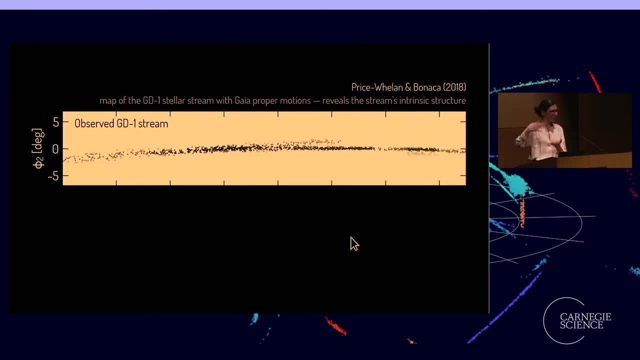 And within a week it was posted on this preprint service, where astronomers announced their new results every day, basically. But then we want to go a step further and see like: okay, can we actually create a structure that looks exactly like this if we impact a stream model? 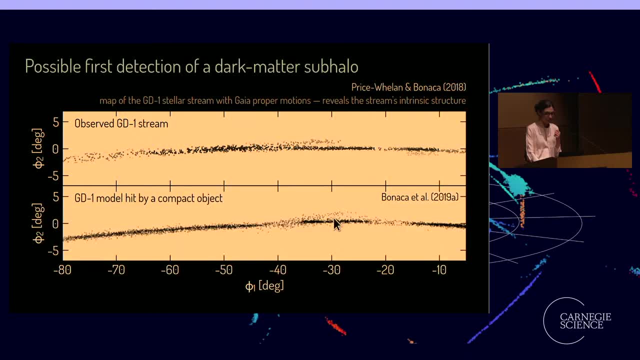 with a dark matter clump or a dark matter subhalo? And the answer was yes, Although you can see from the year, it took a little bit longer to actually produce that comparison properly, But once we hit this GD1 model with a pretty compact object, 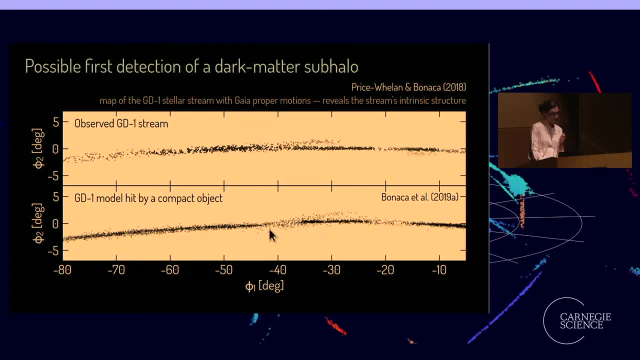 we're able to produce this gap around minus 40 degrees that has the spur of stars that are kind of coming out of the stream, And so that was a success, meaning that, like the impact well, could produce this, And this was possibly the first detection. 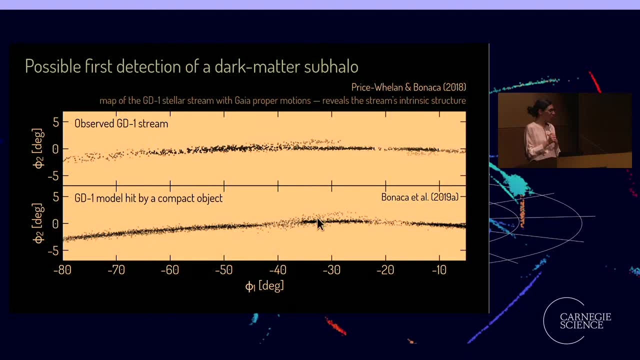 of a dark matter, subhalo, But of course we don't know for sure. It could be some other kind of object, other massive compact object And weirdly enough, this our measurement was completely consistent with there being some rogue black hole orbiting the Milky Way halo. 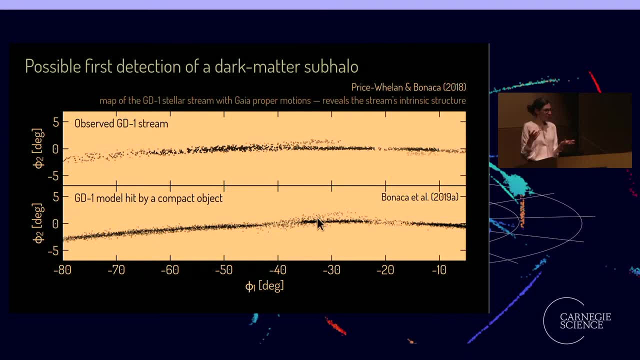 and it impacting it. It's impacting the stream. We don't think it's very likely that there is one, or the odds would be very low, but there could be, And so we thought, okay, what is the next thing we can do? 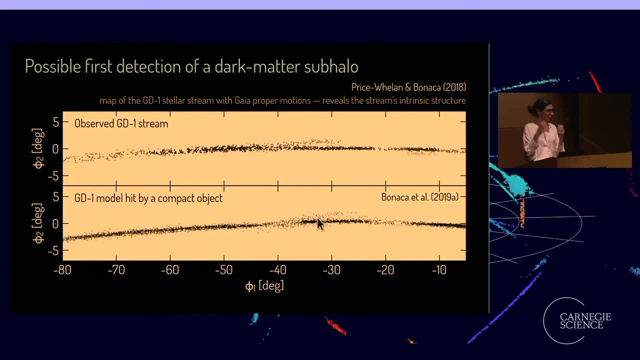 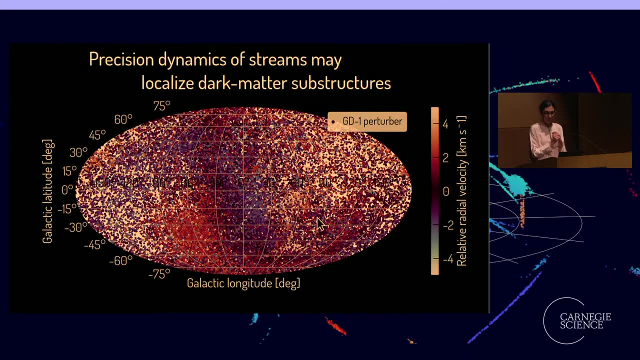 Well, we can try to predict where this dark object should be today and then maybe look for it and see, like if it's really dark. The problem was, when we make this prediction, where it could be. it turned out could be literally anywhere on the sky. 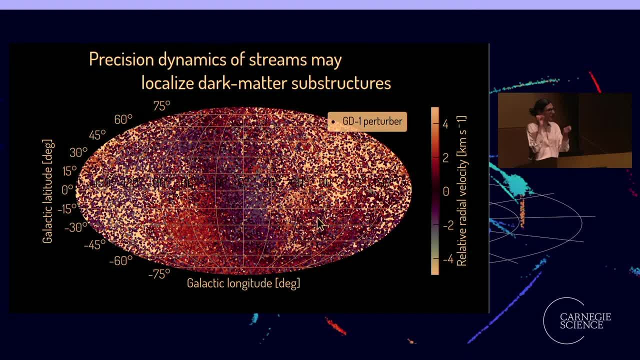 So yeah, the points here are showing like the possible locations from our model. So it was like completely undoctored. We just kind of was creating this kind of simulations of a stream and hit it with different objects or different masses and different orbits. 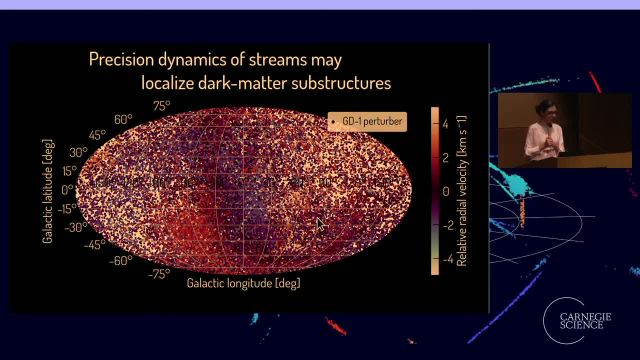 kind of different alignments and kind of predicted where they would be today. And this is where they would be. However, you may have noticed that there is some kind of blue patch and red patches over here And the color bar says round the radial velocity. 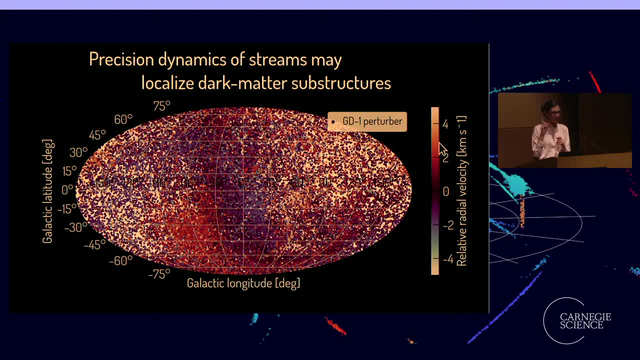 So he's told us that there is some information that we are still predicting something, and that's good, which means that we can test this theory only if we could measure velocities of stars. So then we said like, okay, we should really write a proposal to make this measurement. 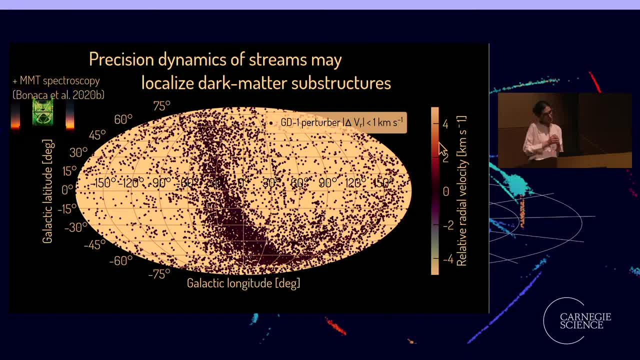 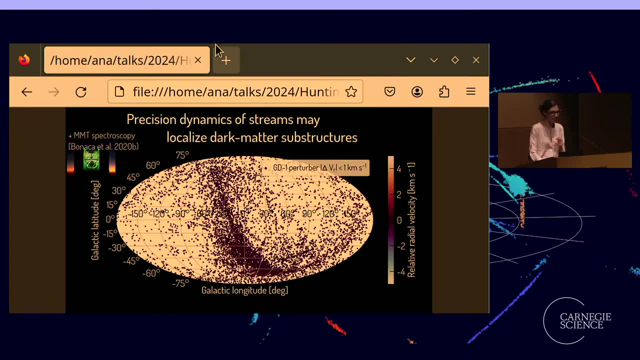 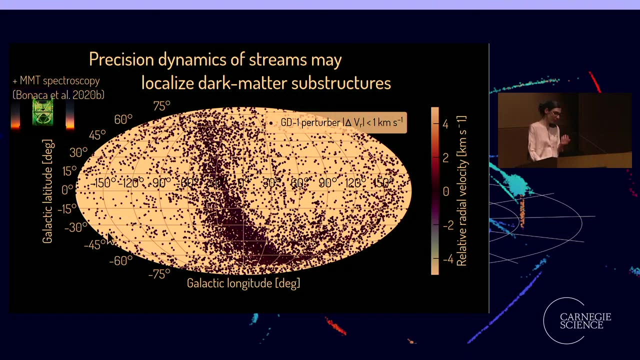 And once we did, we found that there is like very little offset and this different regions of the stream which really narrowed down, well, somewhat narrowed down, where the possible location of the perturber is, And so you can see now it's, I guess it's still possible. 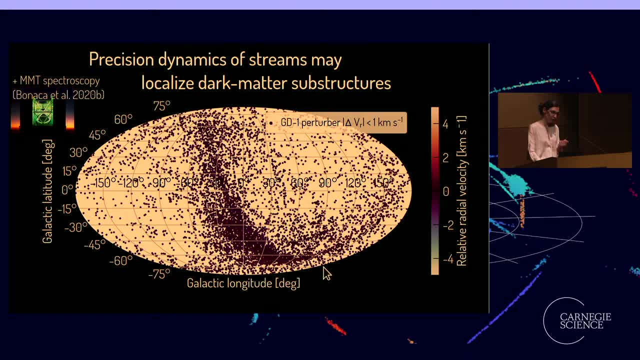 It's like in these regions of the sky, but it's really preferring this one kind of orbital plane over here. We're hoping to do even better And we just received the last of our images from Hubble Space Telescope, like a month ago when we were hoping to measure the. 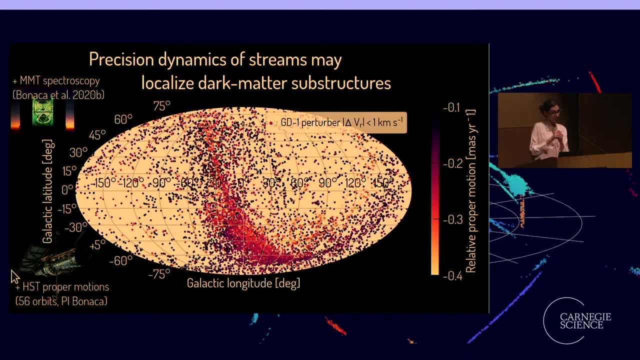 transverse component of the velocity vector to higher precision than what we have now. And now by color coding you can see there's still some variation. So depending on what this measurement is, we may kind of try to constrain this even further and continue our search. 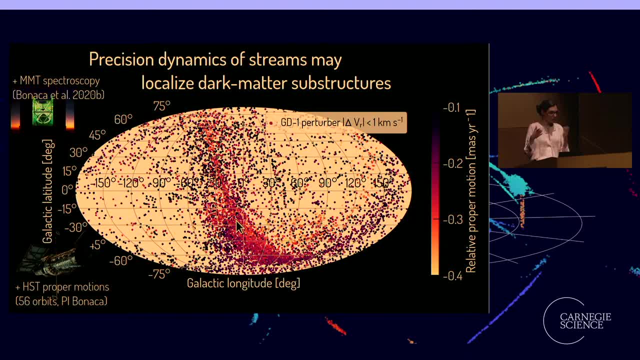 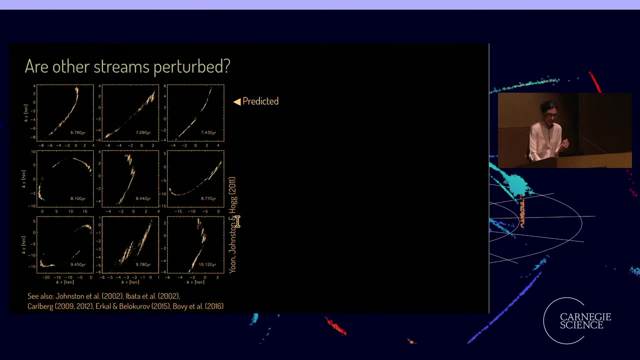 But this kind of is now on hold while we are analyzing the data, and, in the meantime, what we did was ask the question: okay, well, this is exciting. We found we have one possible impact on a stream. How many more should there be? 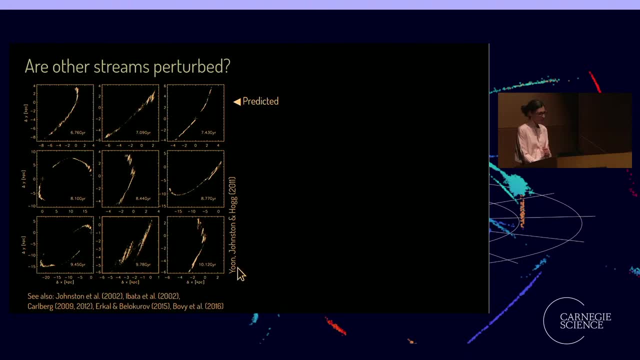 And the answer is lots. So here I'm showing a prediction from 2011 from the Columbia Group led by Katherine Johnson, and Yun was the graduate student at the time. So they were simulating different streams and different orbits and found that many of them, indeed, 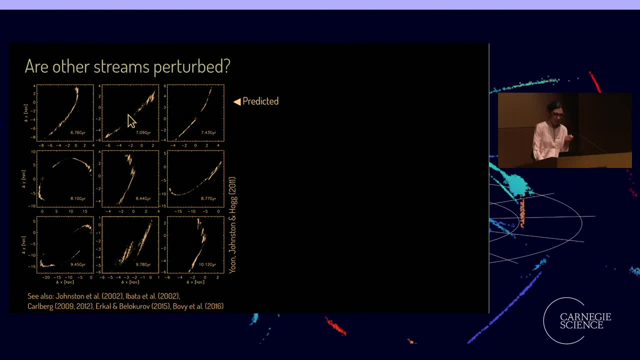 do impact dark matter clumps and kind of the resulting. most streams look pretty different depending on kind of the relative orientation of their orbits. So this was kind of a lot of work when it to predicting kind of how many of these should there be and what should be the structure of streams. 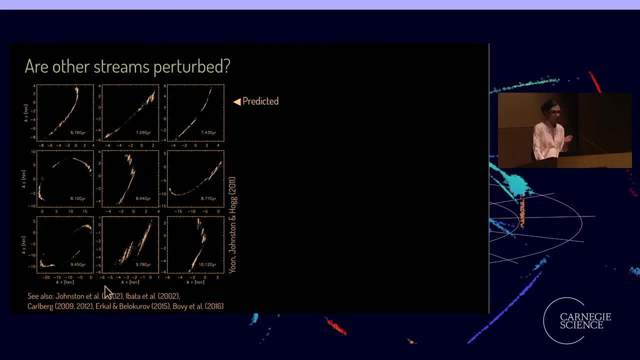 You can see, there was a lot of theory papers on this written And this observation of GD1 really was the first one And it came in 2018, which is kind of like almost a decade later than most of these papers And and really 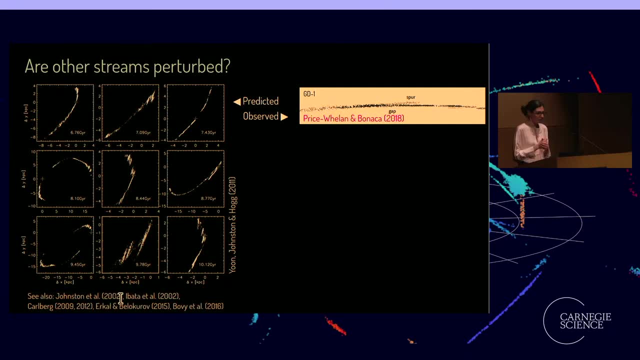 20 years later than the first predictions were made, that we were really first showing that this can actually be done, And so that's really inspired us and other teams around the world to go look into this stellar streams in more detail. So here's one from our own group called JLM. 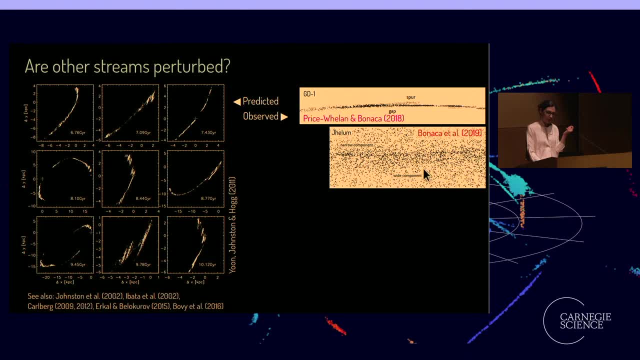 where we found it, has this narrow component and then a broader one. that was not something we would predict in smooth models of the Milky Way. Then there is that same polymer, five stellar stream, that we used so before, but now with much deeper data where we have more stars. 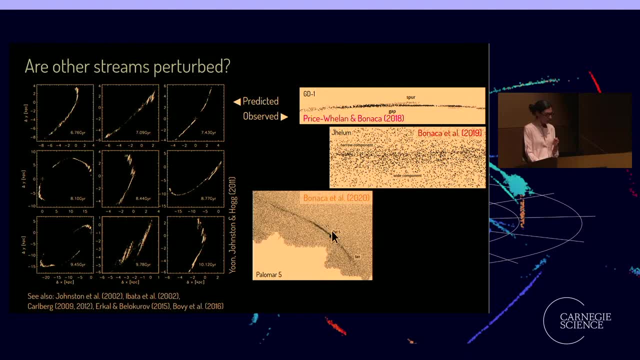 and we start to see that there indeed are what looked like. there are density variations of denser part and less dense part, And then there's even this kind of fanning of the stream on one side, So they're not really equal length and completely symmetric. 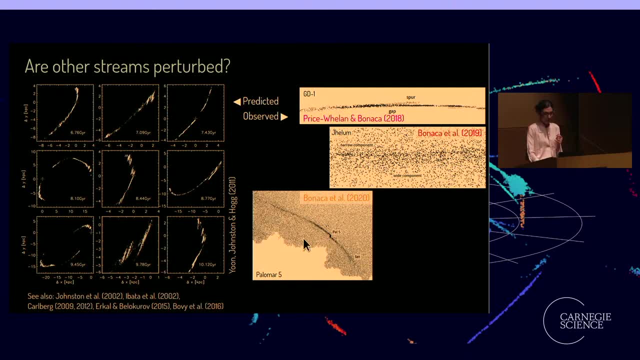 kind of ahead of the cluster and behind it, which is also not predicted in simple models. Then there is this interesting case of the what were originally discovered as two stellar streams, Alika-Uma and Atlas, but then a Carnegie post-doc, Tang Li. 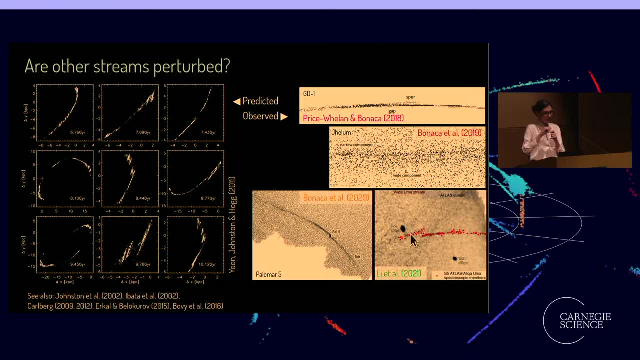 found that they actually have the consistent radial velocity gradient and are probably in the same structure. And then most recently there was this paper from Peter Ferguson, who used very deep imaging data on the stream called JET to find the variations in density and also these kind of weird wiggles. 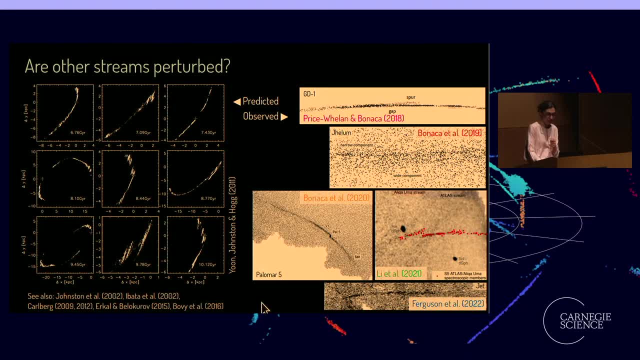 around the kind of along the length of the stream, And so there seemed to be kind of a lot of these structures. So, basically, whichever stream we went to look into more detail, either with this new Gaia data or with some kind of velocity data. 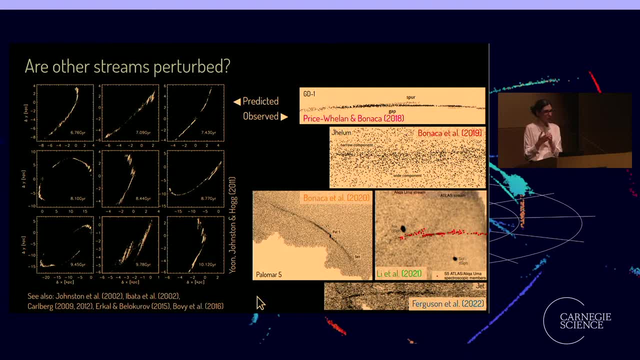 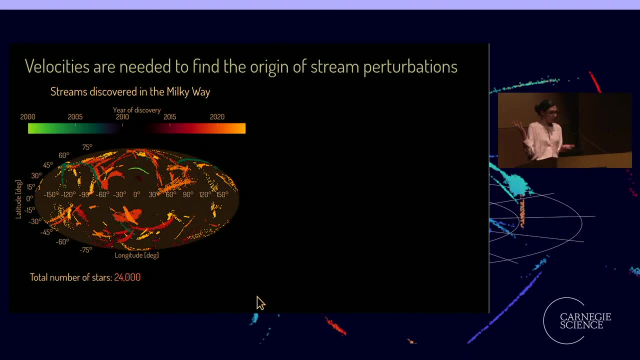 or even just deeper imaging data. we found, like these, deviations from very simple kind of naive structures of what we thought the streams should look like, And there's still lots more to do. So here I'm showing a map, a sky map, of all of the known streams. 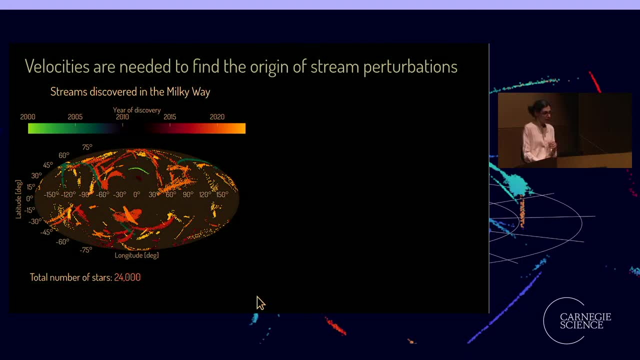 or kind of thin streams originating from globular clusters and they're color coded by the year of discovery. So you can see there are a few ones in this kind of greenish tones that were kind of early discoveries And then there was kind of a lot of new data. 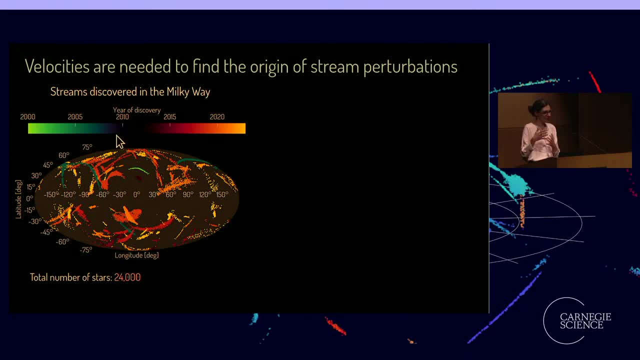 So there was kind of a little bit of a hiatus until really this new Gaia data came along, And then you can see there's a lot of streams that are in this kind of pink and then orange and then yellow colors as well. So in this catalog we have a total number. 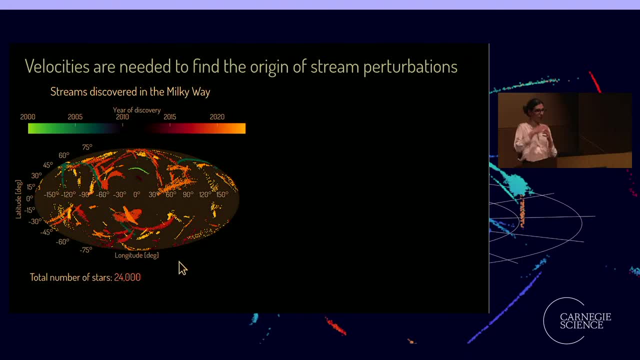 really fascinating number of 24,000 stars spread across almost a hundred streams. Unfortunately, it turns out that stars that have measured velocities- there's only 2000 of them, And we saw how in modeling the GD1 stream and some of these others. 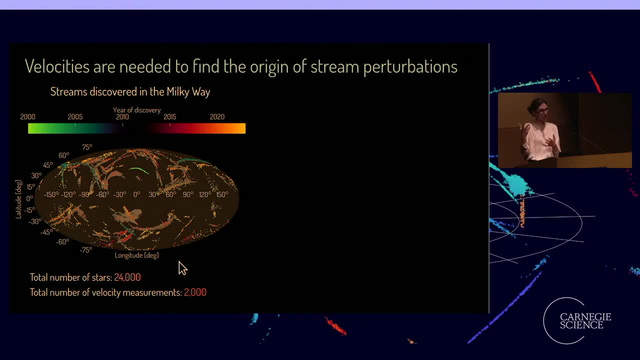 like having velocities is really what is the key in understanding where those structures came from And, yeah, really answering the question of whether it was dark matter or not. So here at Carnegie Observatories we have a lot of telescope time, So my, this Saturday night I'm going to show you. 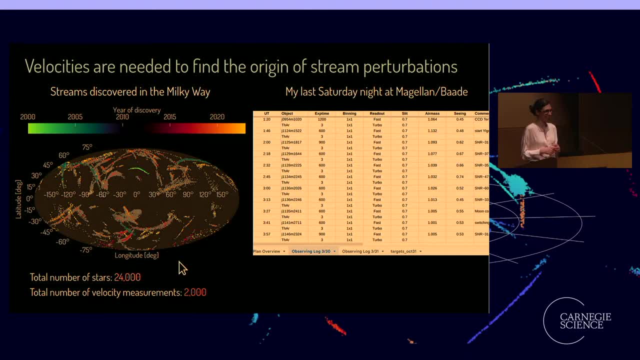 this Saturday night. I'm going to show you this Saturday night. I'm going to show you this Saturday night I was observing on the Magellan-Bade telescope And this is a log, an observing log, from that night. There was a really great night. 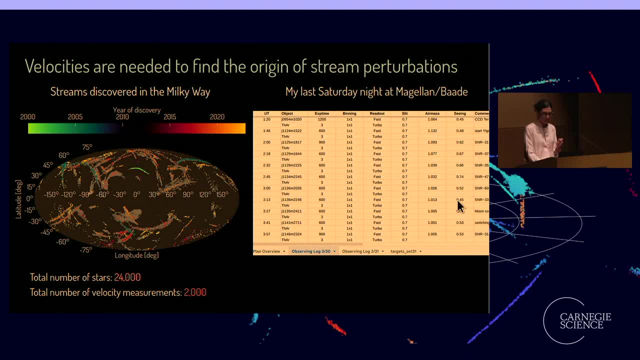 We had excellent weather. for some of the astronomers or amateur astronomers in the room, like the seeing column over here, it's like it's really good, like better than 0.5 arc seconds. most of the time Everything was behaving smoothly. We were. 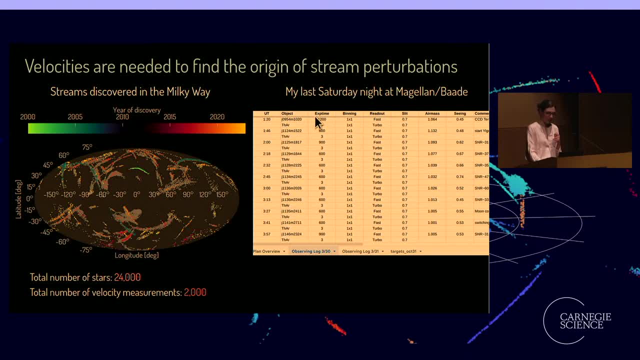 we were. we were observing many stars. The important thing to note is that we were going really fast, So here is the kind of exposure time You can see. it's in seconds, So you can see this like only 10 or 15 minutes, up to 20,. 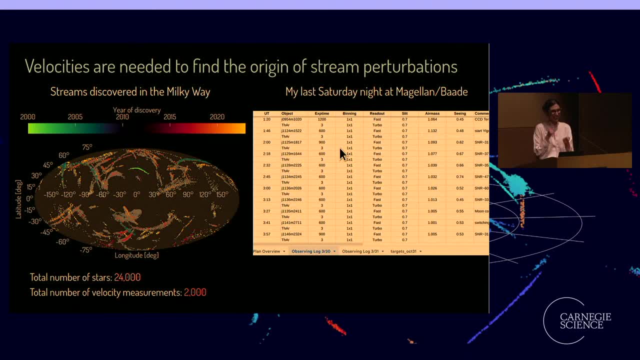 but most were really tense. It was. it was kind of intense, like every 10 minutes switching to the next target and kind of being on top of it all the time. But it was, it was good. We observed 34 stars. 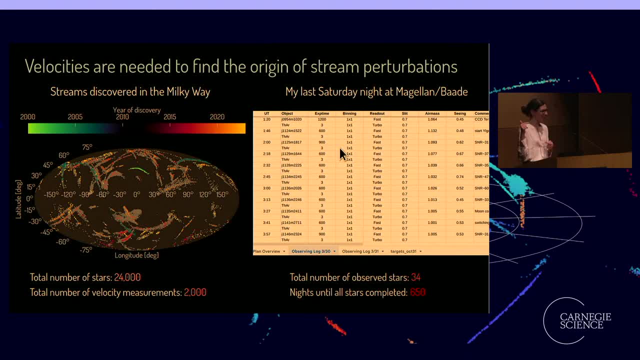 So if you really wanted to go go to the 22,000 stars that are missing radial velocities, it would take roughly 650 more nights. So Carnegie provides its astronomers with a lot of telescope time. This is too much of an ask. 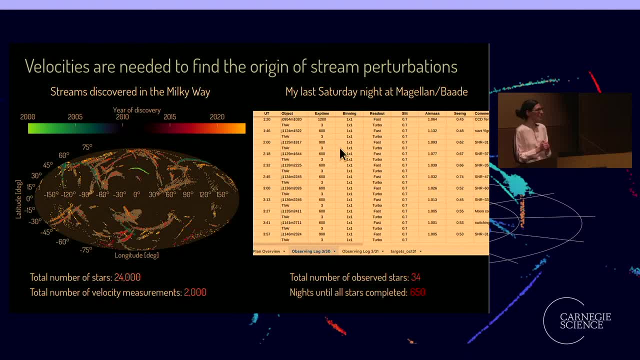 even for Carnegie. So we need to do something smarter, And the targets we observe now are the high priority targets for NASA. So we're going to do a lot of research for one of the streams, but still we're leaving a lot on the table. 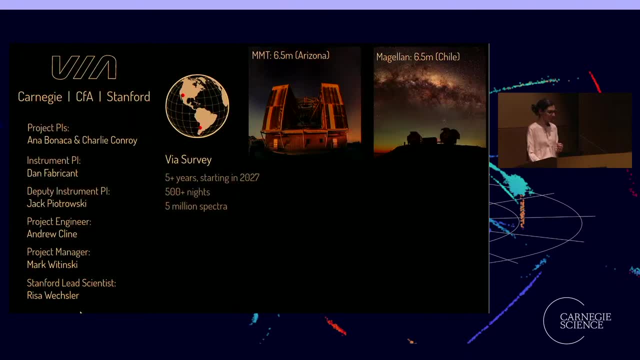 and we really want to do more. So a year and a half ago started a project called VIA that Erica already mentioned- And this is in collaboration with the Center for Astrophysics at Harvard and Smithsonian And Stanford recently just joined- really a few weeks ago. 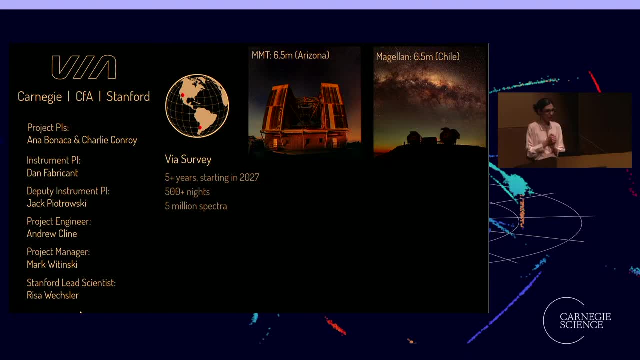 And so the goal of this collaboration is is, in part, to measure velocities of all of the stellar streams that have been discovered in the Milky Way. We'll be running a five-year survey, starting in 2027. out of two telescopes, One is our own Magellan Play Telescope. 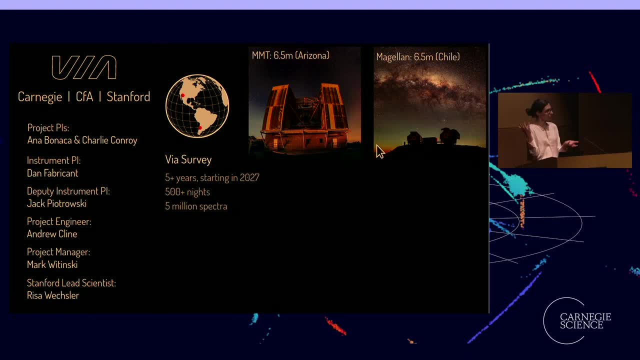 which is a 6.5-meter telescope in Chile, And it will be great for observing all of the Saturn targets. But then we'll also be using the MMT telescope, which is exactly the same 6.5-meter or the same aperture. 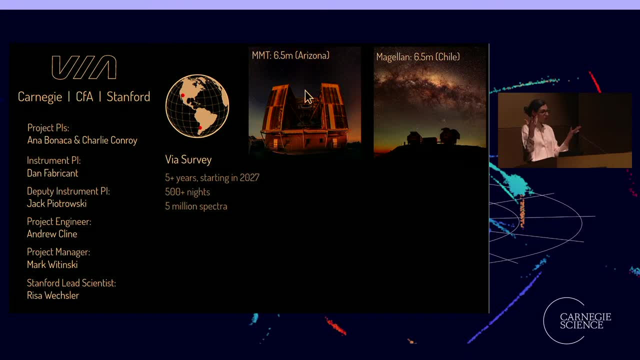 6.5-meter in Arizona. for all of the northern targets, The goal is to roughly do 50 nights per telescope per year, so that we have a total of 500 nights And we're hoping to get 5 million spectra, which is so you know. 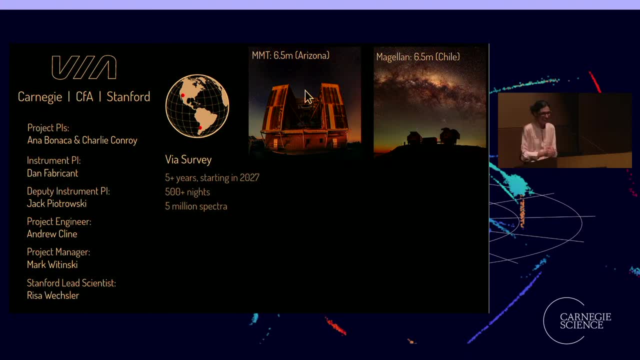 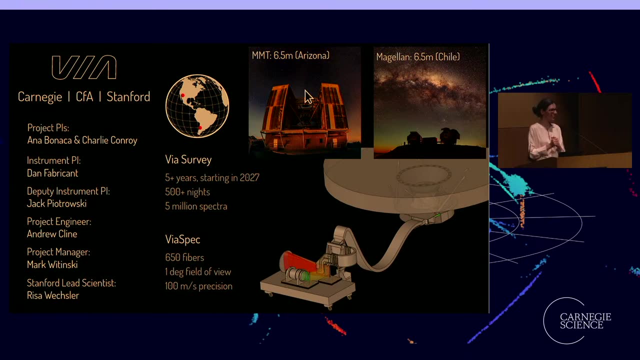 24,000 will be like easy peasy. The problem is that there is no instrument that can do this, So we are also building two new instruments that can simultaneously measure radial velocities of up to 650 stars across one degree field of view, and do this very precisely. 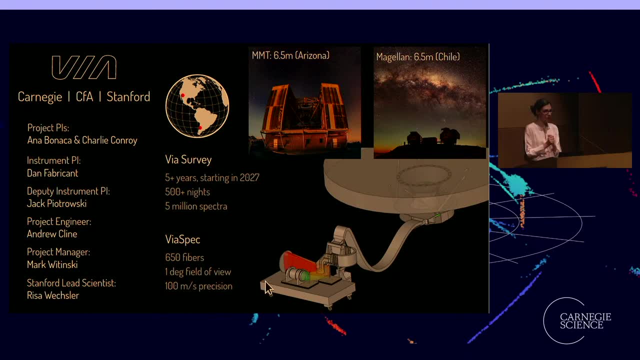 This is really key if we are interested, as we are interested, in pushing for those lower, really lowest, mass clumps of dark matter, because we think still, the velocity kicks that they impart onto the stars will be small. So this is why we are building this new instrument. 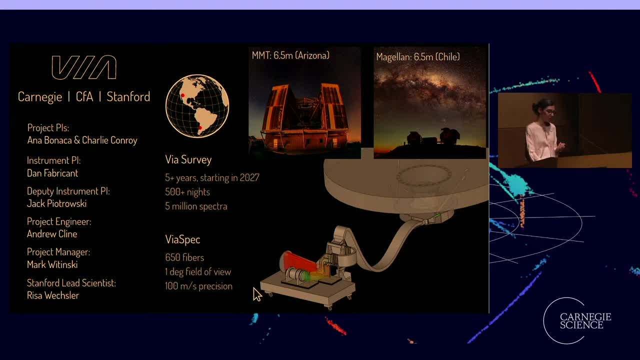 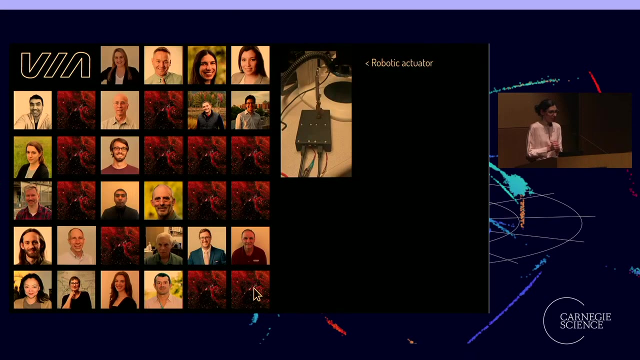 because really none of these instruments that we currently have has this combination of both the field of view, the kind of multiplexing of the number of five objects we can simultaneously observe, and also the precision and sensitivity. When I joined Carnegie I said what I will do, kind of on the theory side. 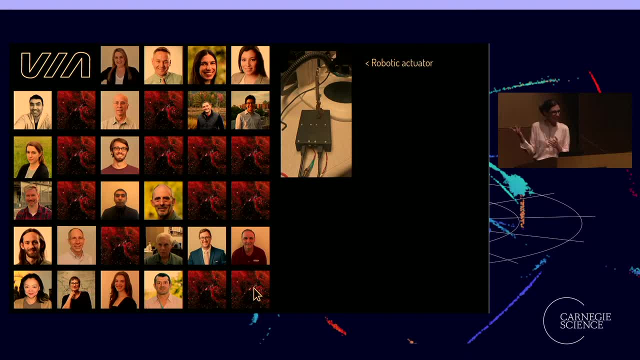 on the observational side. I never imagined I would be part of an instrumentation project, So it's been um a huge learning experience for me and I wanted to show some of the great work that the team has done that I really have just kind of enjoyed. 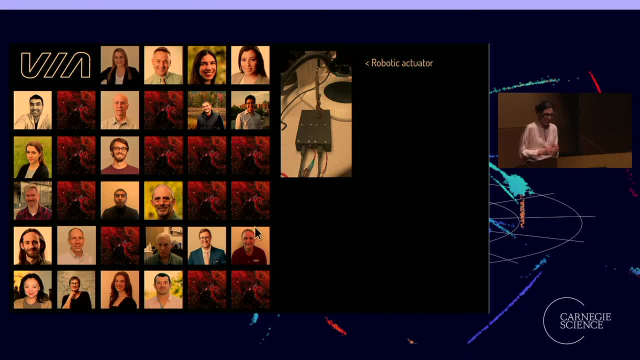 and motivated by this quest for dark matter. So some of the updates from the team will be shown on this slide. So the first one will kind of start from where the light hits the telescope and then will enter a small glass fiber which is kind of 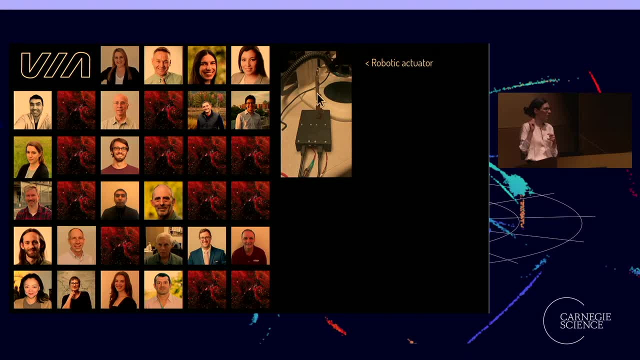 well, maybe if you have fiber internet, it's kind of a similar technology. We're just kind of collecting light from stars. To make sure that, like the fiber is positioned in the right way, we need to- yeah, point it so that it actually is collecting light. 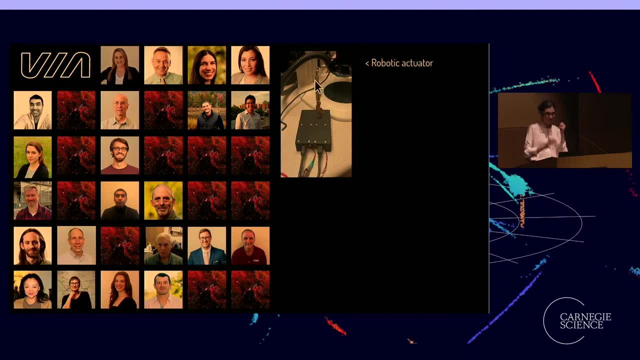 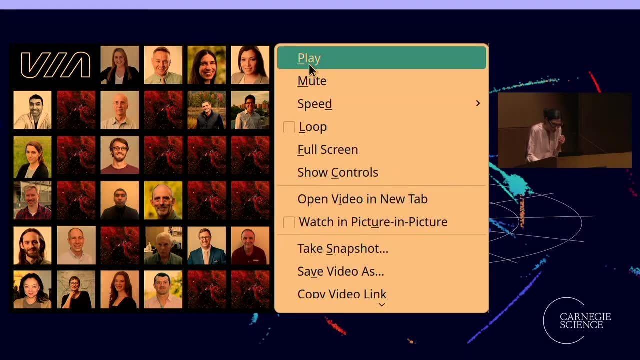 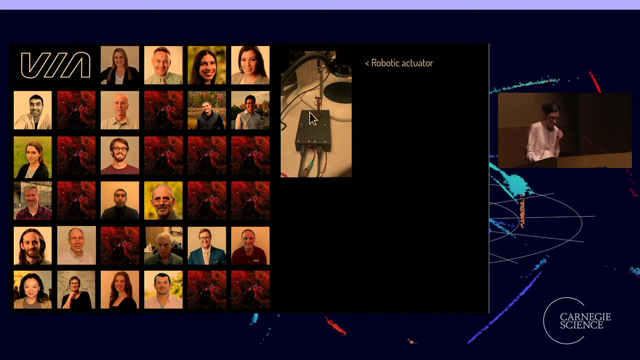 from a particular star and not just kind of blank sky. So what we'll be using is the. are these- oops? robotic actuators That sound a little bit like aliens? So we're working with New Scale Technology Company who produces these actuators. 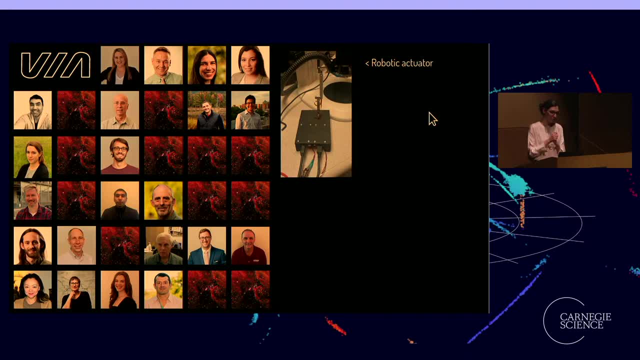 and now we'll be getting our first batch of prototypes in mid-summer and the goal will be to kind of just run them around, like at different positions, kind of different angles, to make sure that if the telescope is pointing towards the horizon or towards the zenith. 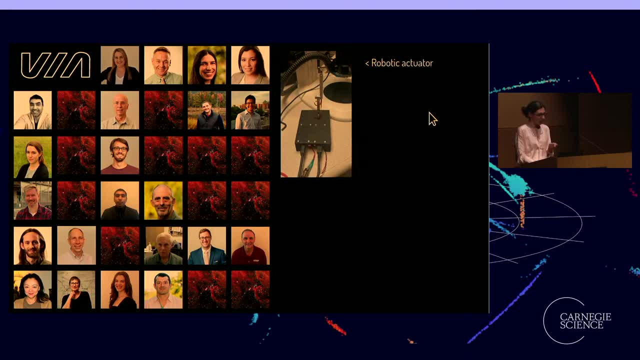 that we are still getting good data. Then, after this light hopefully gets to the fiber that is positioned by this small robot, then it kind of has to go to our instrument where we will be actually measuring this light and the wavelengths of the light. And so what struck me here is that 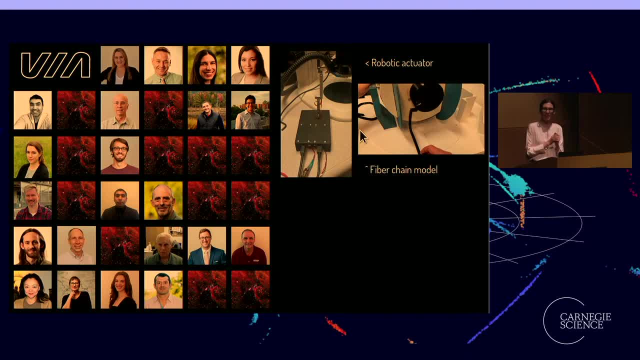 you know things take some time. but things take some time until they're developed. It's not like that. the instrument is just kind of born one day. And this is a particularly fun video that shows a model of a telescope and the model of this fiber chain. 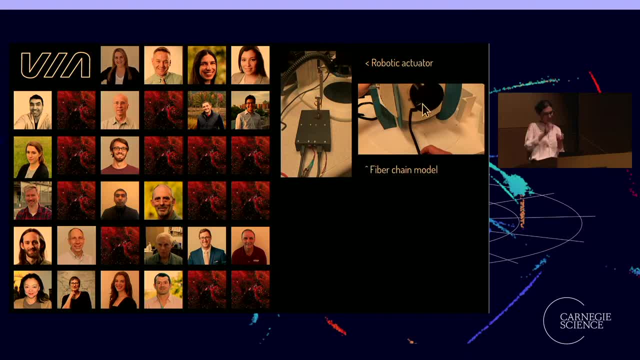 where this glass fibers would be running from the telescope itself to the spectrograph that will measure the velocity. And so you can see we kind of need to make sure we can actually run the telescope All the way. Okay, It's a snug fit for there. 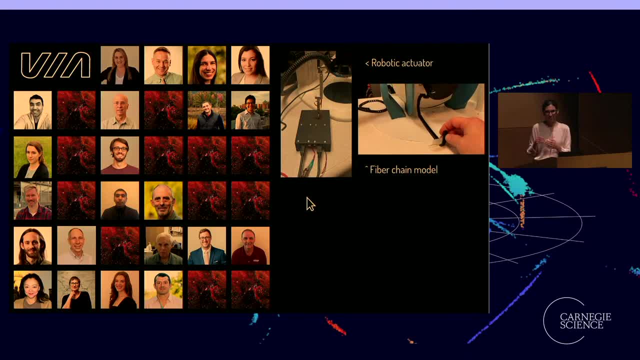 So this is a good way to identify this issue before we actually kind of constructed everything and we're like, oh, we actually cannot go under. So this is very helpful. Then next, kind of as the fiber kind of delivers light to the grating, 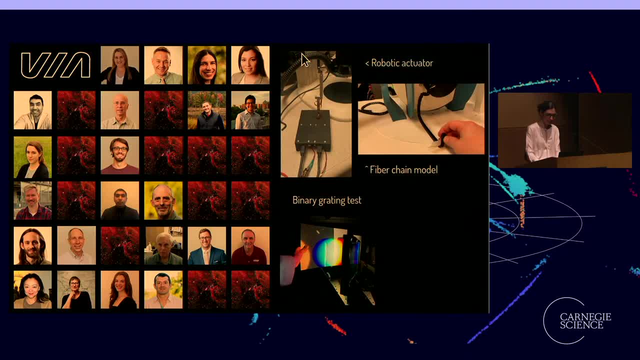 what we are using. Let me take another one. Okay, let's pause this. What we are using here is a new type of grating which is more efficient than what we were using before, And so this is really one of the first times. 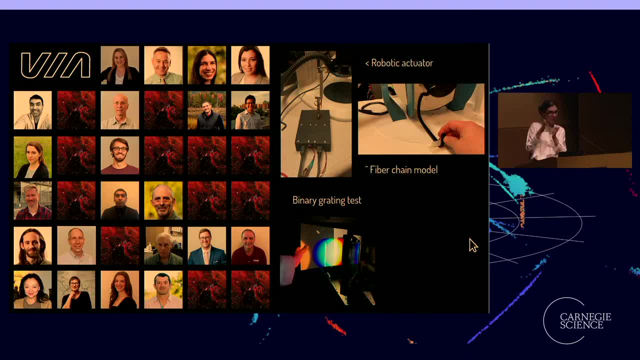 that this kind of grating that disperses the light from, like the ones that we kind of just get from the star, like the any light source, into our rainbow, which is shown over here. We kind of need to test its performance, And this is the first time. 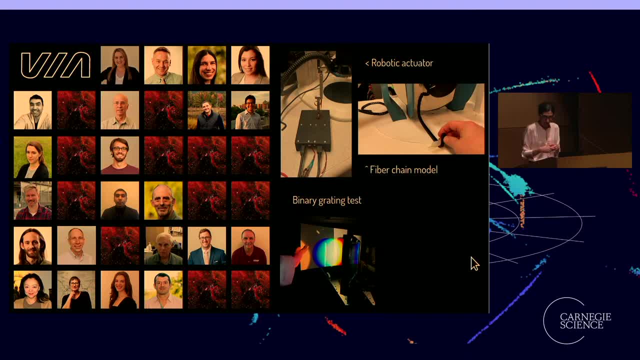 that such a such an element is being used for astronomical instrumentation. So this requires like a little bit of extra testing And then another like kind of final part, once the light is split into this rainbow, into a spectrum, we kind of need to image it. 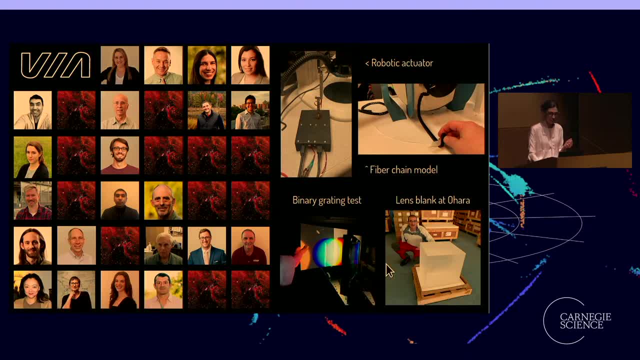 And we just placed an order with the Japanese lands manufacturer called Ohara, And this is one giant block of grating of glass similar to what we'll be getting for our own instrument, And there'll be six or seven pieces that are almost. 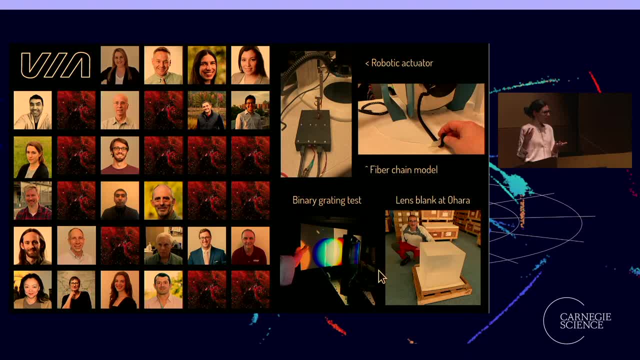 almost as big. And what I learned there is that there are different types of glass. So I originally thought, well, if there is like kind of lenses like in the glasses, it really just matters kind of what shape it is. But no, 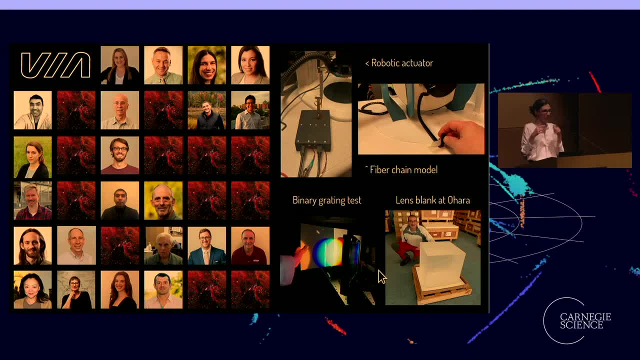 there are even different types of glass, and it also matters and needs to be specified in the in the purchase order, And so it's very, very important to be able to see what kind of glass it is, And so it's been a great learning. 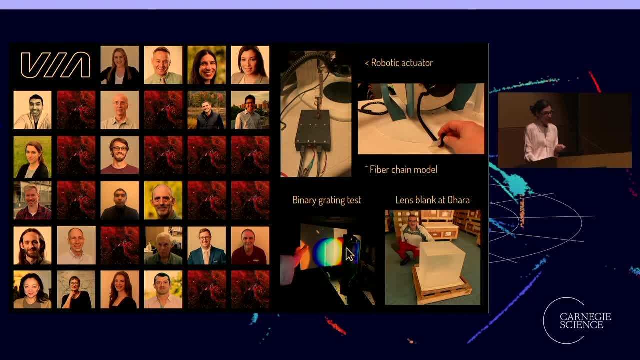 experience and it's been a great team And you can see that there's okay. we're missing some of the photos here, but this is basically what the team is. There are currently 35 people on the roster And you might think. 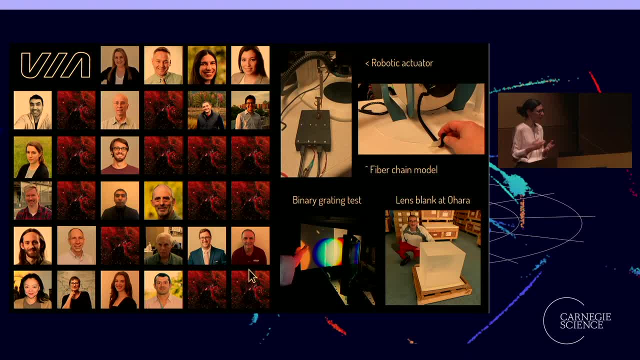 well answering the question: what is dark matter? Doesn't that? wouldn't that require more people? It turns out well. that's the part about astronomy that I really love the most is that small teams can still do a lot of work. 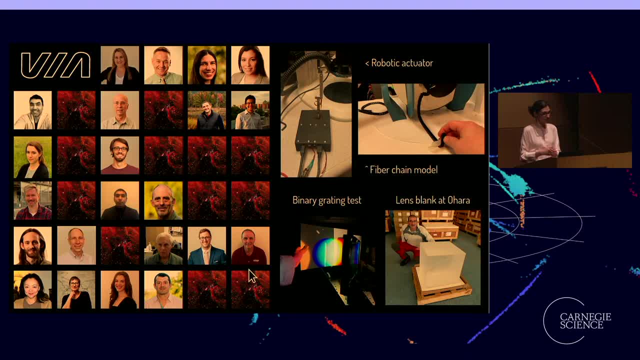 and answer big questions, And the benefits of working in a small team is that we are really close to everyone. Everyone kind of knows what they're doing. I'm learning a lot about this instrumentation, but we as scientists on the team- all are constantly. 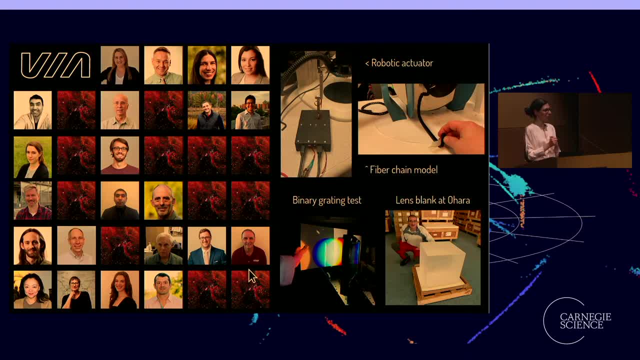 talking to the engineers and saying like, okay, what if we modified like this aspect or change like this particular lens or, you know, properties of this binary grading? How does this affect our final output? And so we are kind of. 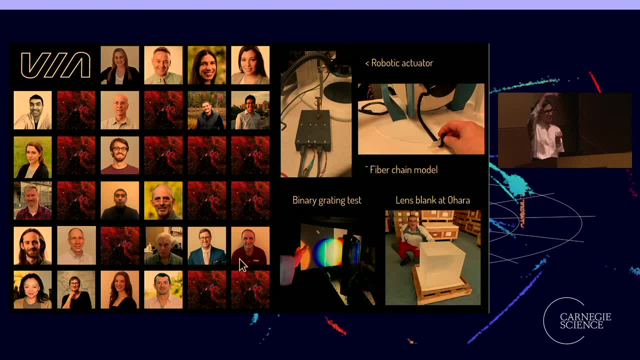 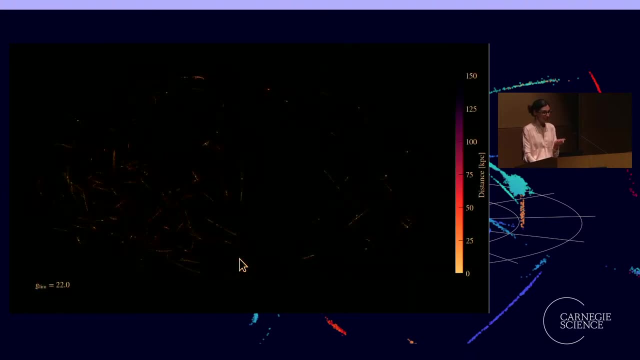 constantly modeling all of this kind of from the light hits the hits the telescope, it kind of to our measurement of the radial velocity And it's super exciting. As I said, we are hoping to be on sky in 2027 to start operations. 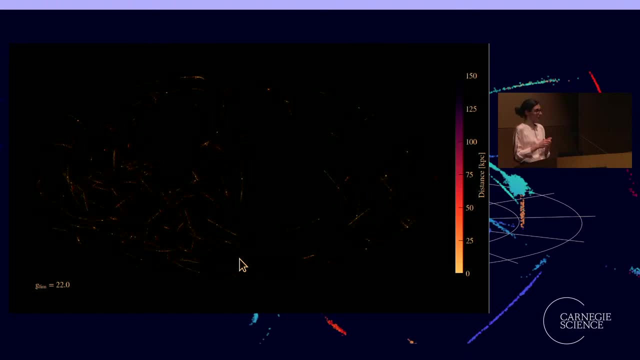 The reason for that is that on the observatory in Chile there will be a new observatory starting to operate, the Vera Rubin Observatory, And this is a giant telescope that will be creating a well fully taken, full image of the sky. 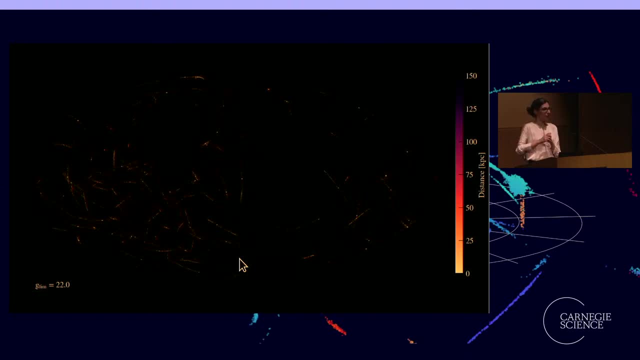 every three nights, So there will be a lot of faint stars detected there, And we expect that our view of the stellar streams will transform. Here I'll be showing a simulation of a set of stellar streams, So this is kind of 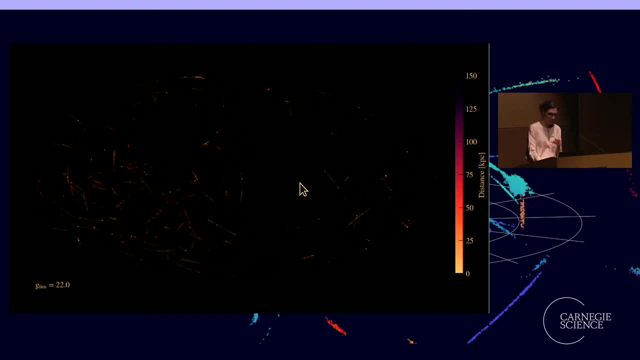 artificial data, but something that we might expect kind of to see today. And you can see the coloring is by distance And most of these are kind of yellowish. They're nearby, So the limiting magnitude is 22nd As LSST. 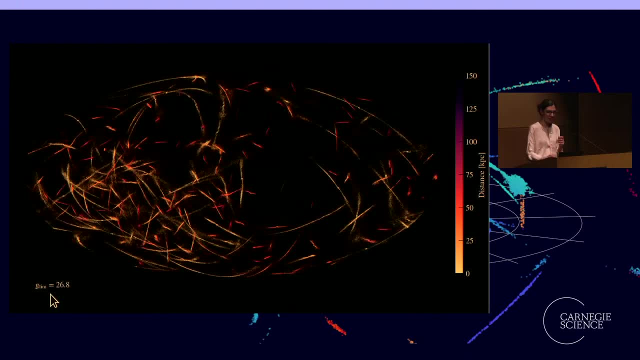 plays on. you see, this magnitude increases And there are so many more streams. The nearby ones are like a cocktail And we even see some of these very distant ones, kind of almost to the edge of the galaxy, more than 100 kiloparsecs. 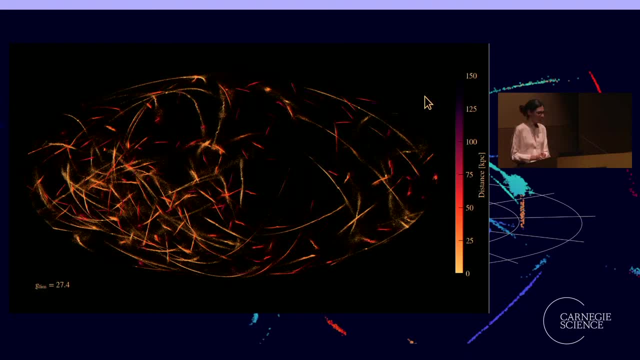 away. So this is what we're hoping to map with VIA, measure radial velocities for all of these stars And then maybe in five, no sooner than that, I guess in three years- I can come back and tell you more about. 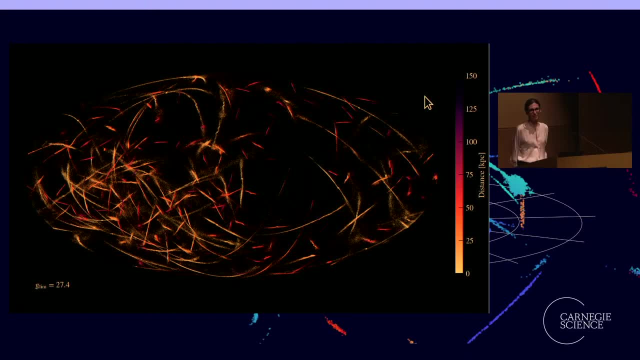 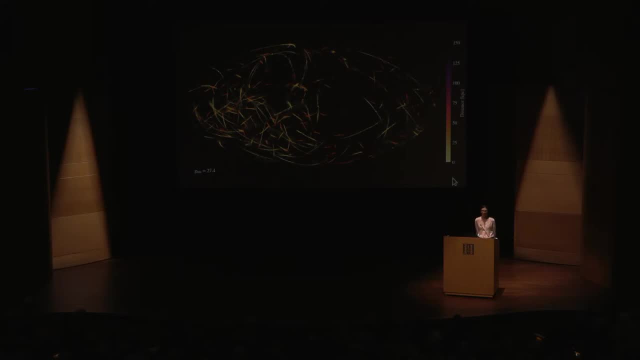 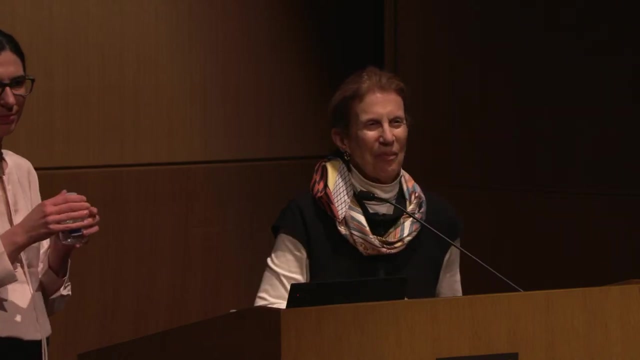 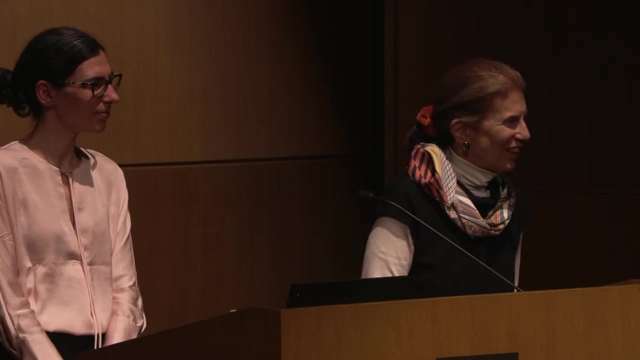 this, Thank you. Thank you so much, Anna. We have microphones at the back in the transverse aisle there And people are welcome to come up and ask Dr Bonassa questions. Please do Great talk, Thank you, I was. 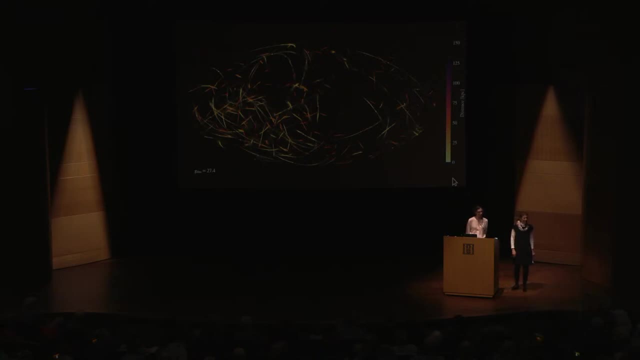 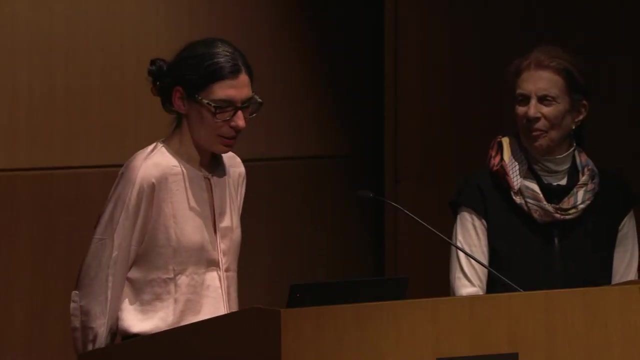 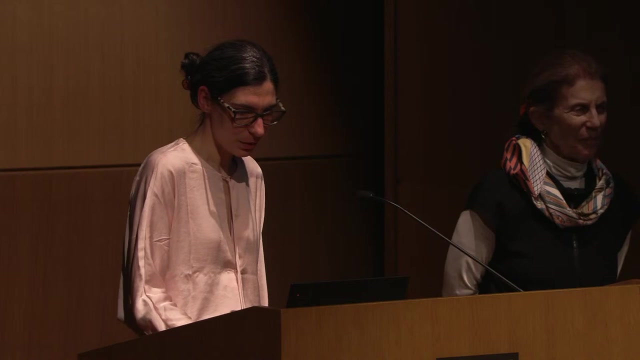 wondering if you would be able to gather additional data if you were looking at different wavelengths of light and what that could potentially provide you. Yeah, that's a great question, So a lot of what we've gathered from creating maps like this. let me